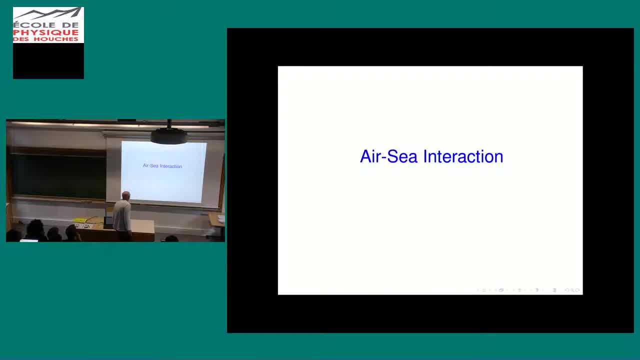 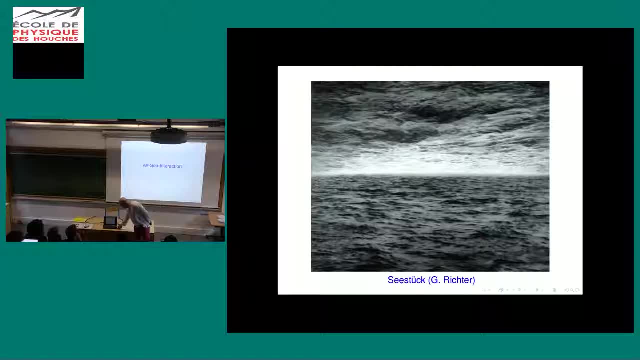 About my work. So the title- the first title- is a little bit complicated. What I'm really talking about is AFC interaction And, for those who have been to my office, this is the painting- a poster of a painting- which is hanging in my office. 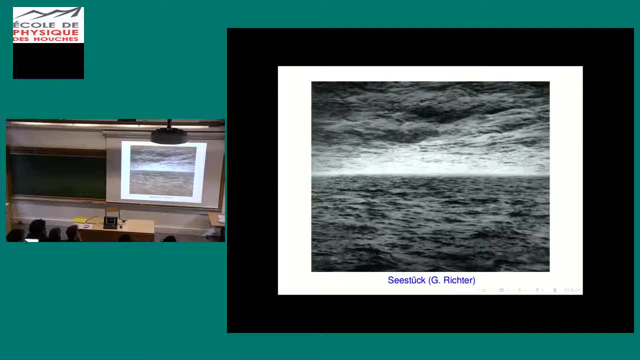 It's a painting from Gerhard Richter. He's probably the most selling, best-selling painter, living painter, German painter. And it just means part of the ocean And it shows- for me it shows very well- ocean-atmosphere interactions. 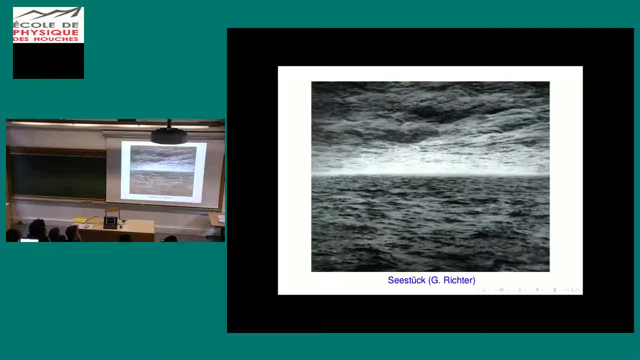 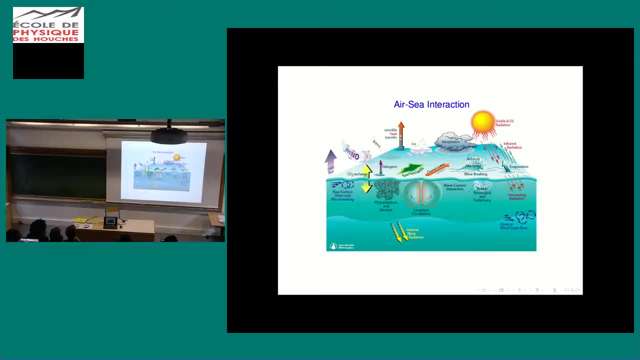 You have the ocean, you have the atmosphere. Both look turbulent and looks a little bit scary too. And so well, I like this painting very much. And this is another drawing of AFC interaction which is a little bit more scientific. 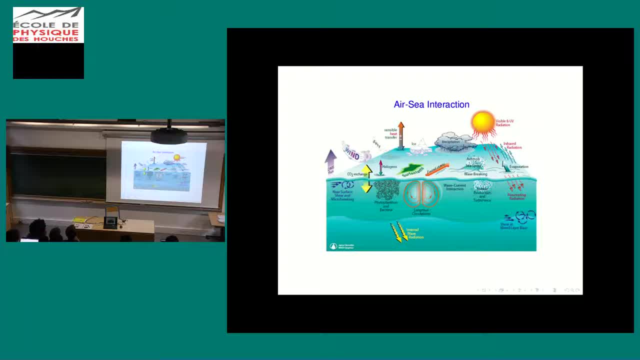 It comes from Woods Hole Institution of Oceanography and it gives us an idea of what is really going on at the ocean-atmosphere interface. And today I will talk about only one process which is happening, and this is here: the wind stress. 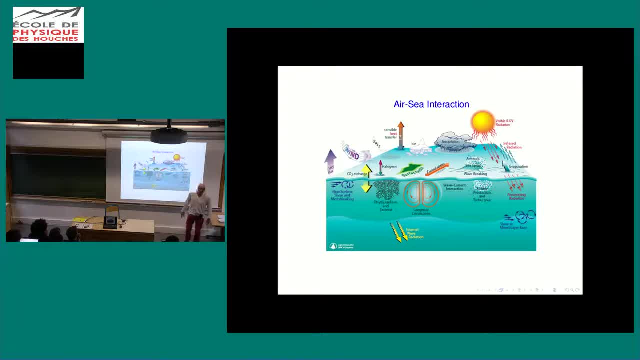 So the wind imposing stress on the ocean, because if there is wind blowing above the ocean and if the ocean current and the wind's velocity are different, then there is some shear and there is some interaction. Of course, when both move at the same velocity then there is no shear, but when they have different velocities then there is a shear. 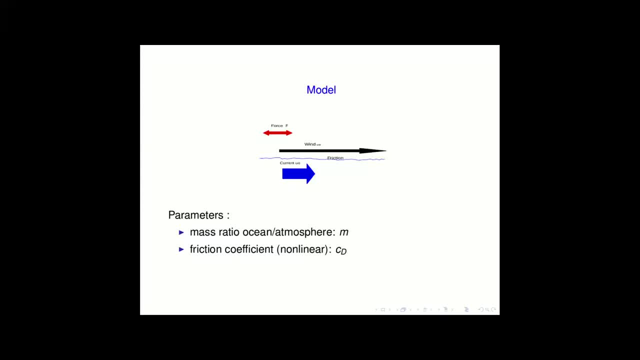 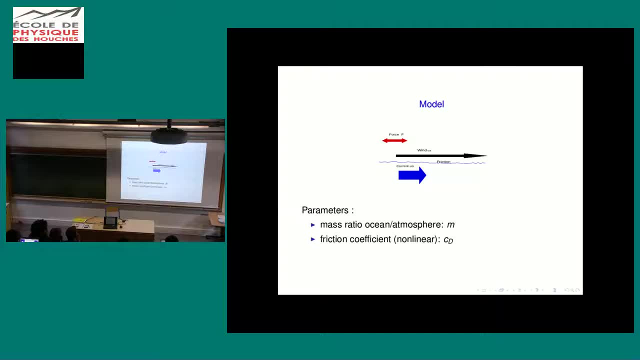 So this will be the essential of my presentation, And so I will just talk about a very, very simple model. It's a very idealized toy model, so it's kind of idealization type one, So it's very. I mean, I start from a very simple model, then I make it a little bit more complicated. 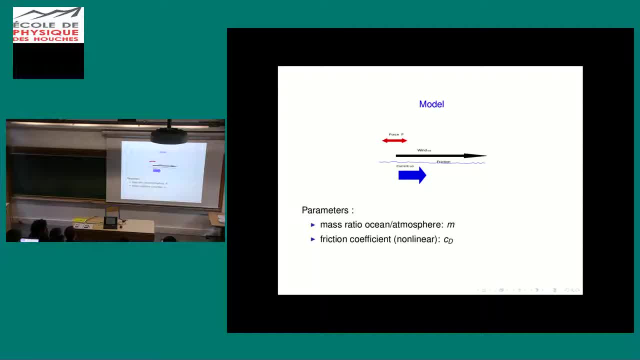 And then I look what it can teach us. these simple models can teach us about models which are a little bit more complicated. So I have The ocean, which has a current, and I have the wind which is blowing above, which has a wind velocity. And there is friction in between. So there is one thing which is important is, of course, the ocean has more mass, so the density of water is much higher, And then the wind, so there is a mass ratio between the ocean and the atmosphere. 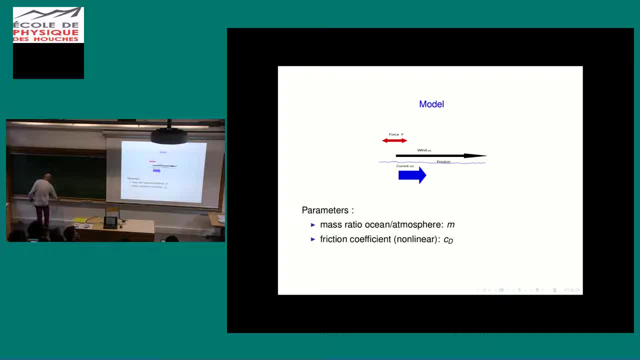 So the atmosphere above and the ocean below. So I'm looking at a slice of the interface, a slice of the atmosphere. So this would be the atmosphere. Then here the ocean, and the ocean layer is much it's thinner than the atmosphere. 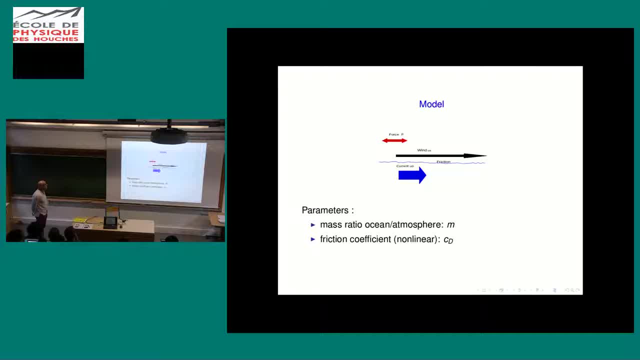 So I have a ratio between this ocean mass. so, per unit area, the ocean mass and the atmospheric mass, which is m, is chosen in most of my experiments to be equal to 100.. So it's just a number. And then there is another very important parameter, which is the friction coefficient. 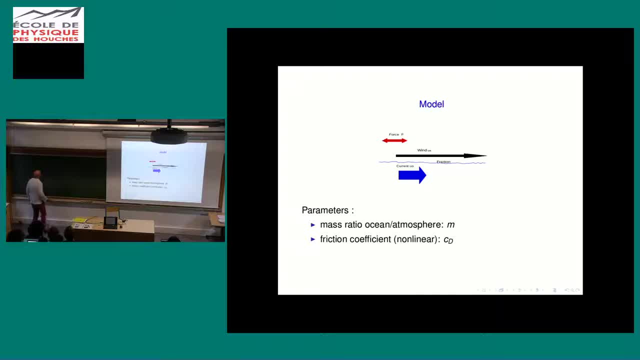 So I use nonlinear friction. during all my talk I will use nonlinear friction. So the friction force per unit area in my models is always given by this friction coefficient, this drag coefficient, times atmospheric density, times US. So what is US? 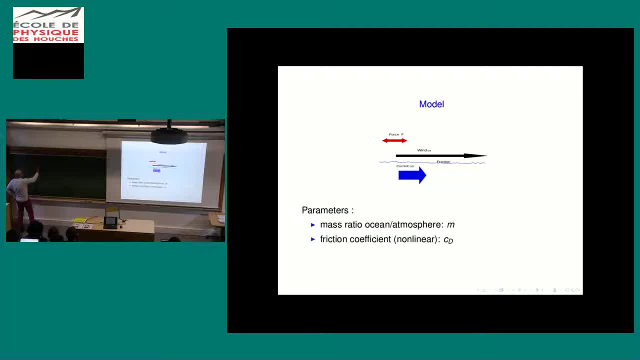 US is just the difference between the atmospheric and the oceanic velocities. So I'm looking at the difference in velocities between the ocean and the atmosphere. It's not- I mean, it's not not everybody does this- You, in former times, when people considered the shear which is applied to the atmosphere, 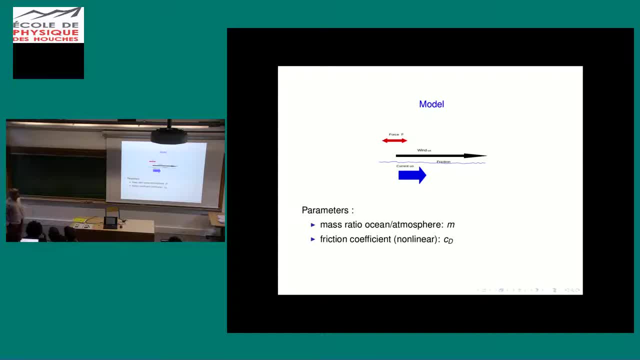 to the ocean from the atmosphere. often in simulations, only the atmosphere atmospheric velocity is considered, And the ocean velocity, which is much smaller, is often neglected. So I don't, I don't do this, I have always the shear. And then of course there's friction. 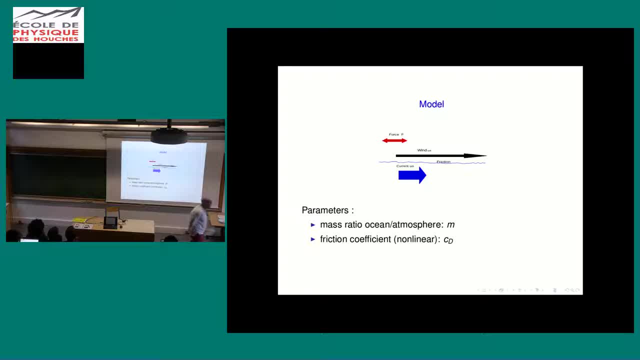 So there is depletion of energy And this depletion of energy, I need some driving force. So I force the atmosphere. The atmosphere is forced by some type of forcing And this keeps. actually, this is the forcing on the atmosphere, only on the atmosphere, which keeps the system going. 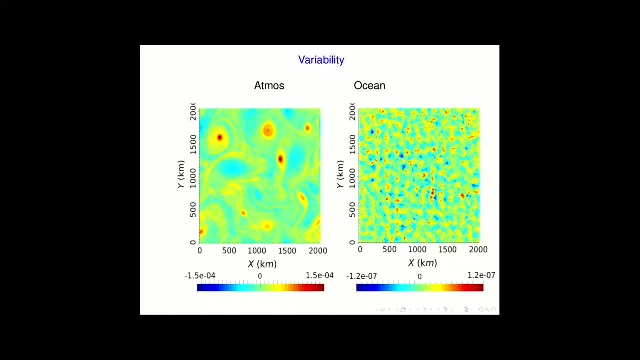 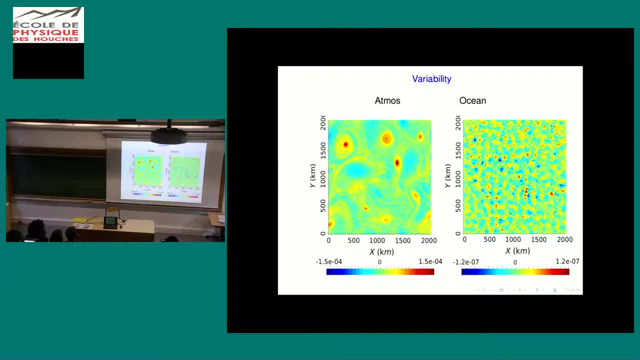 And so I'll have three slides of motivation why I do what I do. And this is the first slide. This comes out of a work which was done, which I did together with a PhD student of mine, Amy Moulin, where we looked at the same problem, just in shallow water. 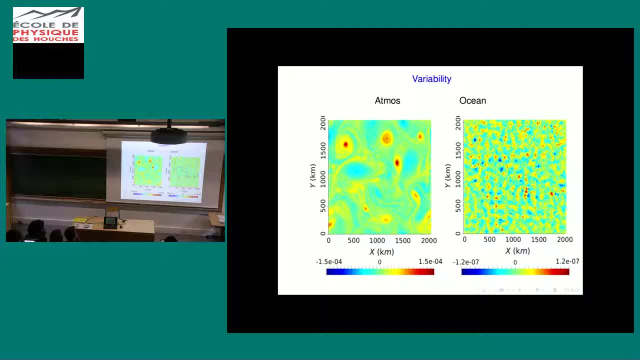 I won't explain why shallow water, But we had a shallow water model for the atmosphere, We had a shallow water model for the ocean And we had them interact only through friction. So there's no in all what I say today. there is no heat exchange. 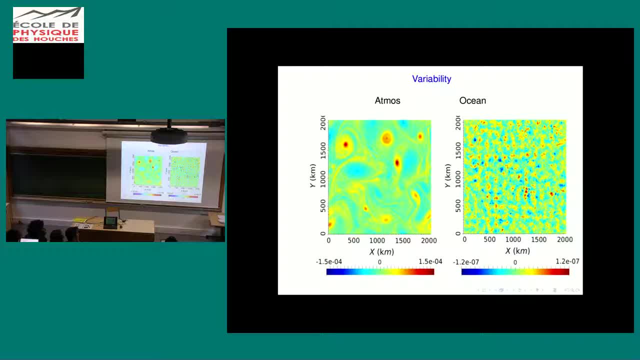 I know that heat exchange is very important, But I'm not talking about it today, And what we had actually is this configuration. So this, what you see, is vorticity. This is on the F-plane, shallow water, This is vorticity in the atmosphere. 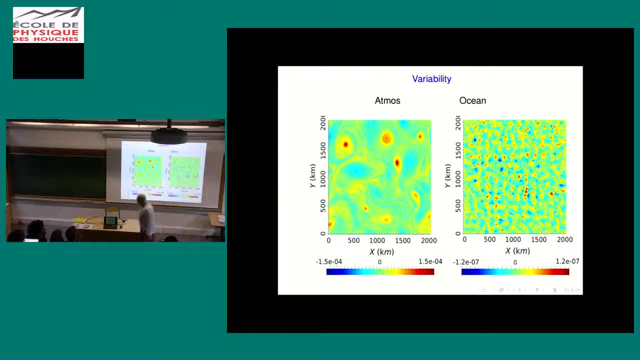 This is the vorticity in the ocean And it's biperiodic in the horizontal directions. And then what we had is we had a grid of of of four by four, of four by four cells, And in every cell this forcing was the same. 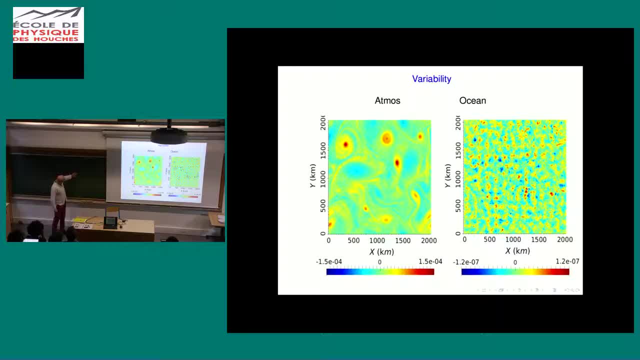 So it's periodic, And so there is this same forcing here, here, here, And so there's this periodic picture And the system is periodic in also, in the all the all, the system is periodic And this is what we saw. 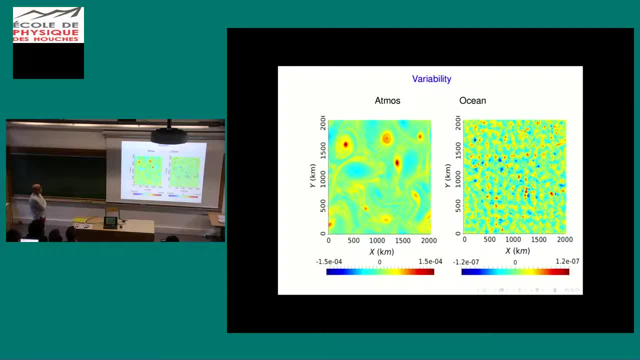 So here we have a rather small friction coefficient. CD is 10 to the power of minus four. And what you see here? you see the turbulent atmosphere And you don't really see the forcing in this snapshot. If I would show you an average over. 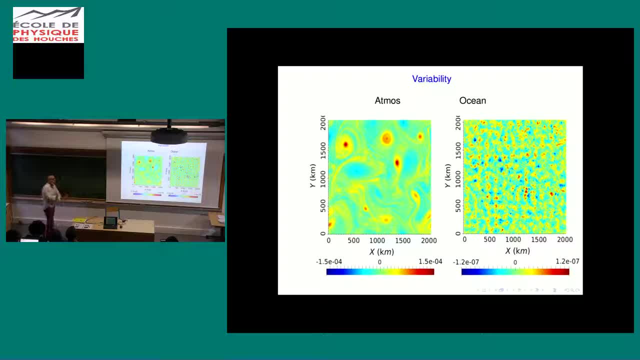 over a long period, then the forcing, of course, would appear. appears, But you don't see it in an instantaneous snapshot due to the turbulent motion, And the same is somehow true for for the atmosphere, And the same is somehow true for the ocean. 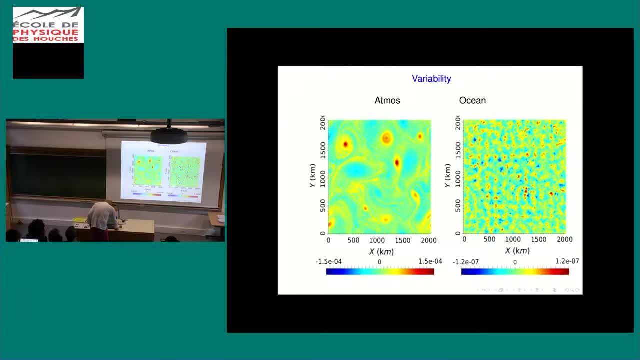 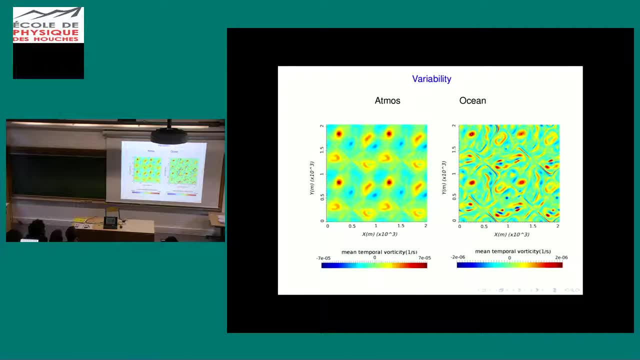 as you can see here. And so then, what we increased, we did. we increased the drag coefficient and showed and wanted to see how things changed quantitatively. But finally we saw that there is a, that there is a qualitative change. So how is the forcing actually? 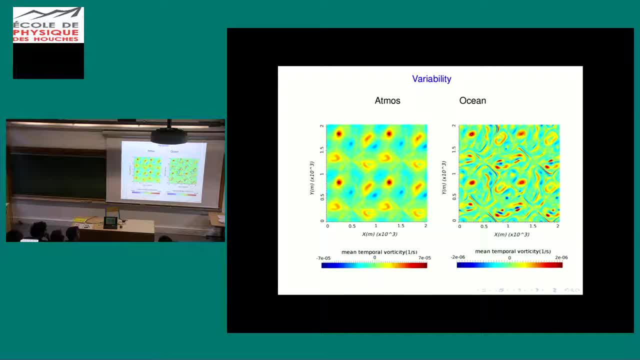 I mean it's a deterministic forcing on your, on your boxes, on your Yes, So the forcing is only on the free surface. So what we actually do is we have a free surface which is in shallow water, And we project the actual free surface on the forcing pattern. 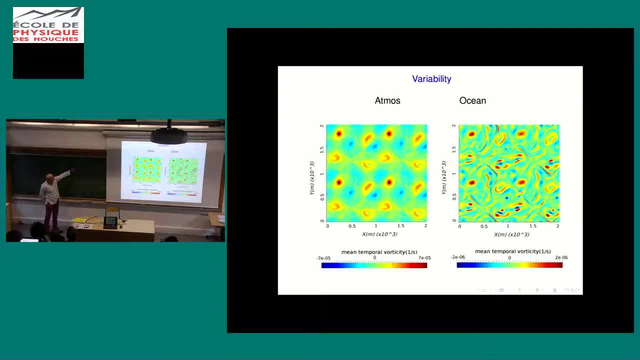 Then we look at the difference And then we add the forcing pattern so that it is, it is restored, so that the forcing, the mode of the research pattern is restored to the imposed pattern. So this is like if you have a, if you have a. 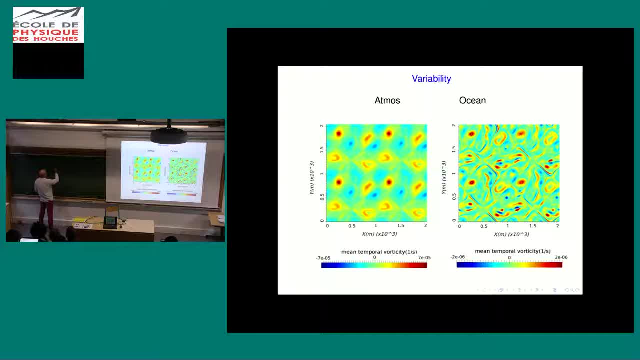 if the forcing would be just a- let me be more precise- if the forcing would just be a, a sign function, then we kind of do a full. we look at, we look at this mode in the solution, And if the amplitude of the mode is too small, 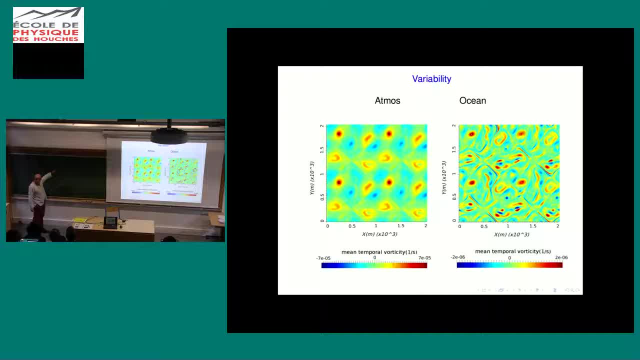 we increase it. If it's too high, we decrease it. So this kind of forcing effects only the forcing pattern, the forcing mode and all the other, all the other dynamics is unaffected by this, by this type of forcing. It's actually equivalent. 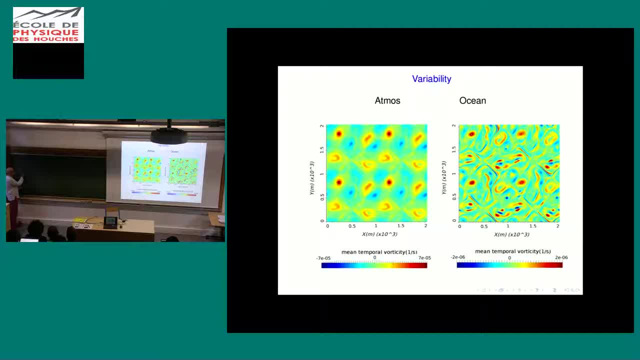 So if if people look at flow through a tube, sometimes they impose the through flow and they keep it, they keep it constant, And so the the transport and it's. this is the same thing, It's just we don't impose the through flow. 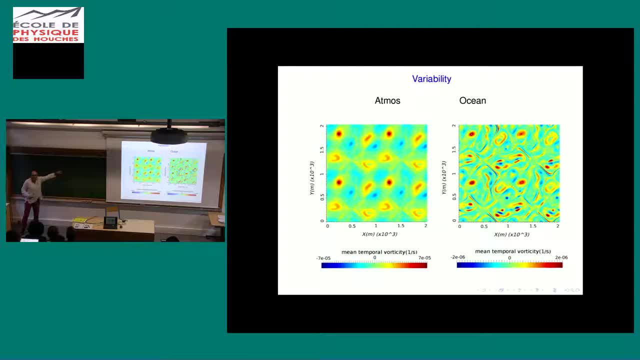 but we impose the amplitude of this of one mode with the forcing mode actually. So that's what we do. This is a nice way to inject energy in just one mode and to leave the other modes unaffected. They are direct, not directly affected by the forcing. 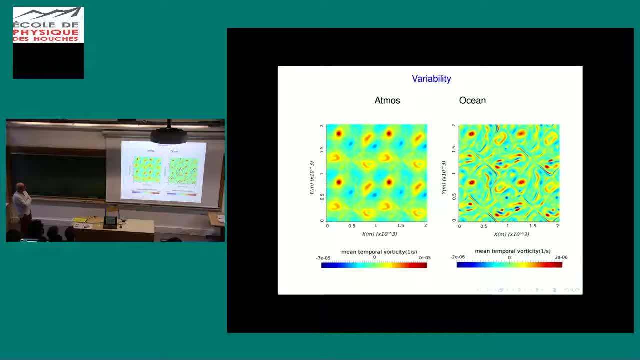 And so we did this also for this higher with higher friction coefficient simulation, And what we saw was something very different, because we saw this picture And this picture did not involve involve in time, So it was frozen, We didn't have any time evolution. 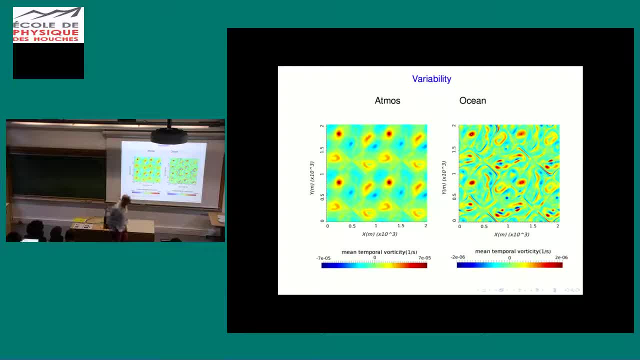 So what we have is here: we have some spatial variability, but we don't have temporal variability, because if there weren't spatial variability, then the value here would be the same here, here, here, in all of these 16 squares, But this: 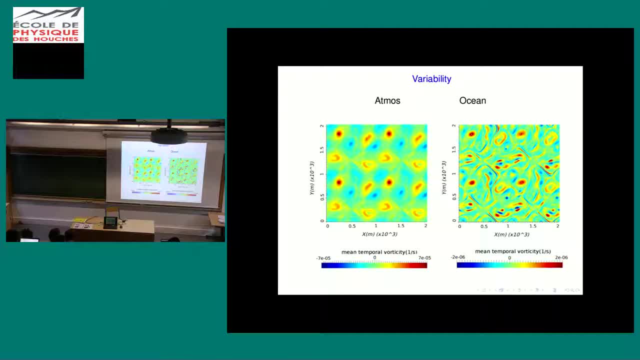 that's not what what happened. And so for the lower mode, for the lower- sorry for the lower- friction coefficient, we had temporal variability, And for the higher friction coefficient, we actually had only spatial variability and no more temporal variability. 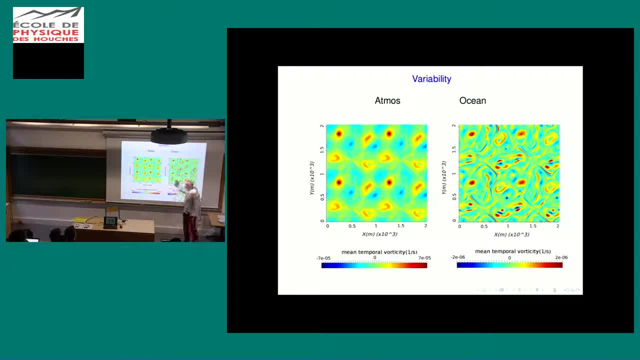 And this is true for the atmosphere and the ocean. So they don't, almost don't evolve in time anymore. They are, they're frozen, but they're not frozen in a periodic, in a periodic way. Yeah, Sorry, So I'm not sure of the equations you're solving. 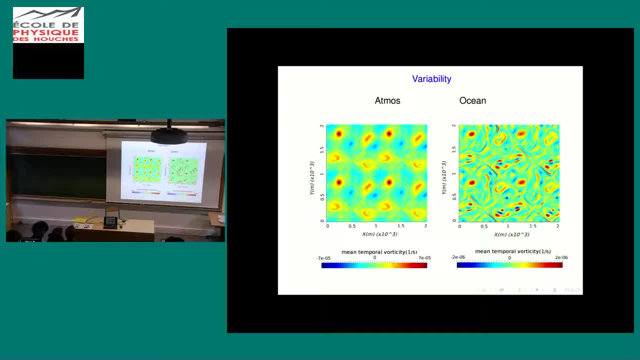 So it's two shallow layers, Yeah, two shallow water layers. So the interface can be deformed between the ocean and the atmosphere. Sorry, Can you deform the interface between the atmosphere and the ocean? No, no, it's flat, Okay. 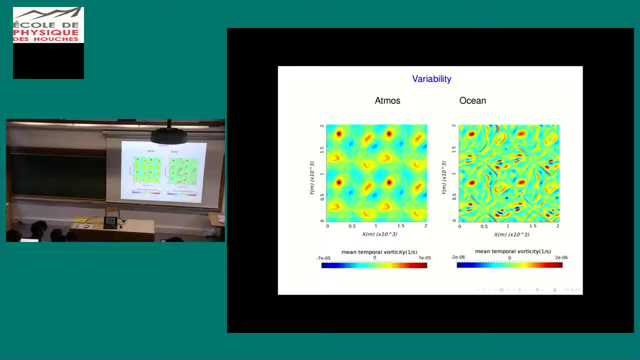 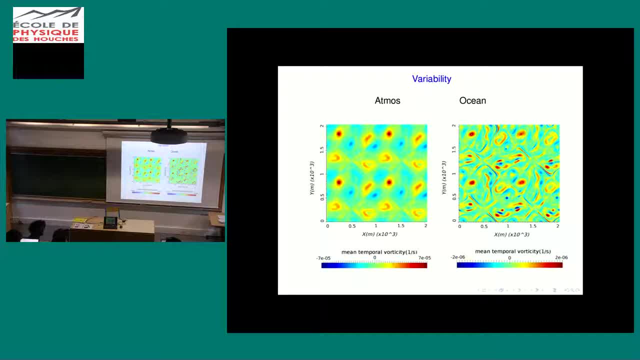 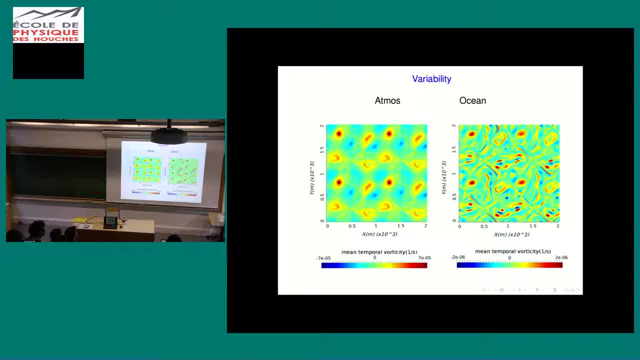 Yes, Okay, Thank you. This actually was very important remark because of course, the ocean velocity acts on the atmospheric velocity. some features tend to appear repeatedly, like, for example, in the atmosphere plots. you see some very similar structures as different cells, but, like for the ocean, 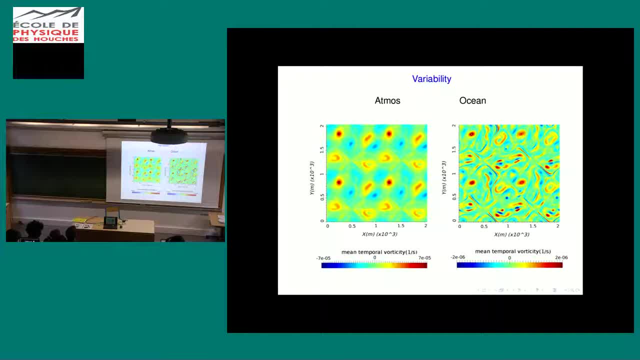 I see some more differences among, like, the cells. so what causes the difference? so it's not completely periodic, neither in the atmosphere nor in the ocean. so, as you said, there are differences. where this differences come from, I don't know. I mean it's not so, then we 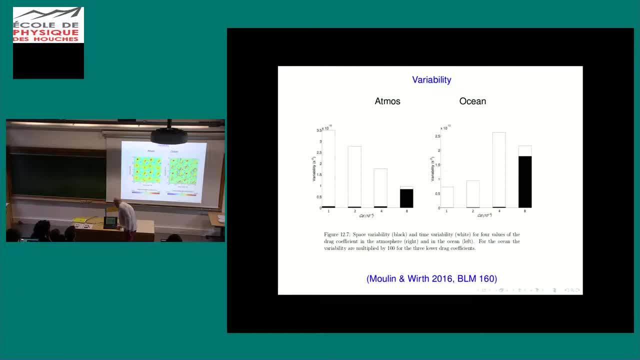 try to quantify this and to quantify this we actually what we looked. we we separated the variability in spatial variability and temporal variability. so for the spatial variability, we just calculated the average over all this 16 squares and we also turned it by a 90 degrees, calculated the average, so we had a an ensemble of 4 times 16, 64, which is of 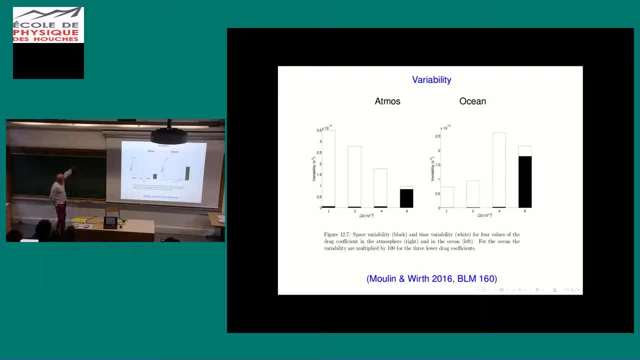 course not independent all this, but this way we could really calculate an average cell. and then we looked: what was the difference between this average cell and 16 cells which are present here? and then we also looked at the temporal variability. that is, we looked over several integrations of a long time and we looked at the variability in time. and the result is what? 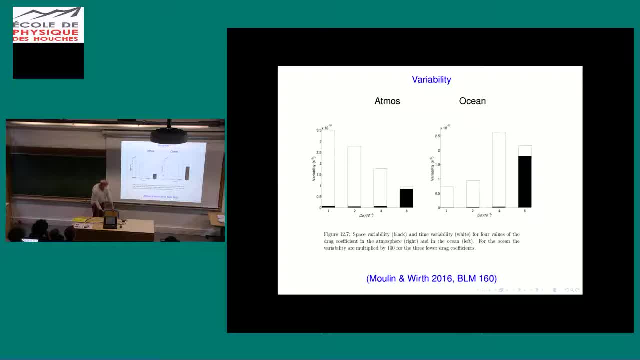 you see here is that for the lower friction coefficient, there's no longer any kind of what you actually see is. so this is the total variability, what is white is the temporal variability and what is black is the spatial variability, And what you see is that for the lower friction coefficients, 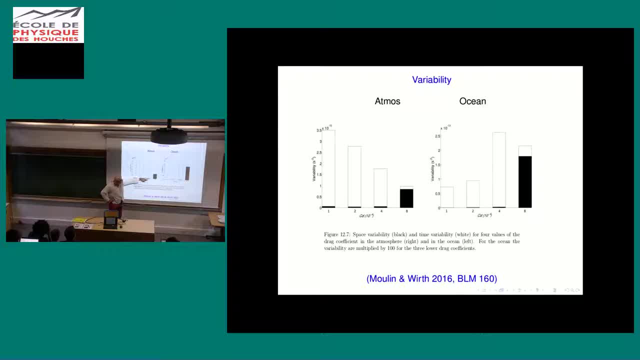 actually we don't have almost nothing. no spatial variability. So if I would show averages for the low friction drag coefficients, then the averages would be completely periodic in space, whereas for the higher one, spatial variability is almost degrees to zero. sorry, temporal variability is almost degrees to zero. 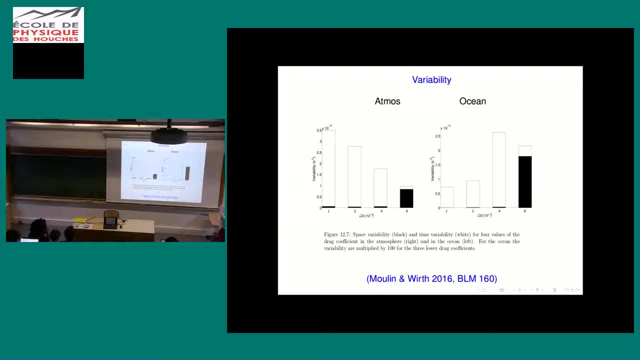 and everything. all the variability is in the spatial part, so it's completely frozen. So this is something which we observed, which happened, and so what we thought about is that this might be well question. Just to be sure, by variability you mean the variance. 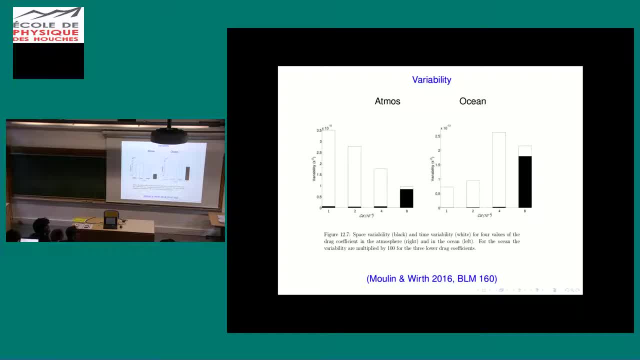 The variance? yes, yes, yes, Okay. and why is that second to the minus two, if it's a variance of velocity? We looked at it in vorticity. Ah, vorticity, okay. So all the plots I showed were vorticity plots actually. 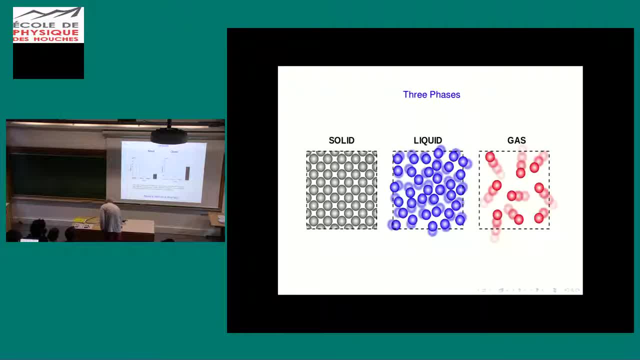 Okay, And so this resembles somehow what is known in condensed metaphysics, class transition. And so, to explain this, let me show two slides, or three slides, about the class transition. So when I was in high school, I was taught that there are three phases to matter. 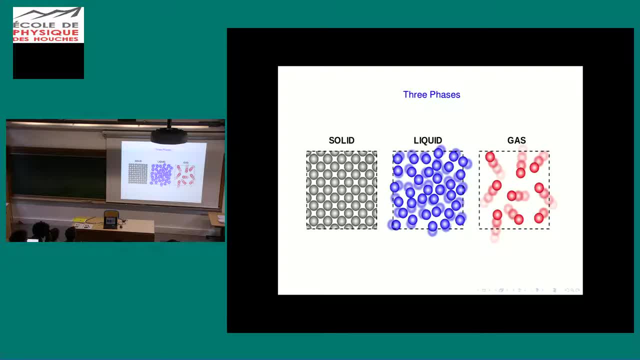 gas, liquid and solid, and if something is solid, then it has a crystalline or ordered structure like you see it here. This is taken from the Internet and this is how to explain the three phases of matter. However, if you look at the solids which are around us, 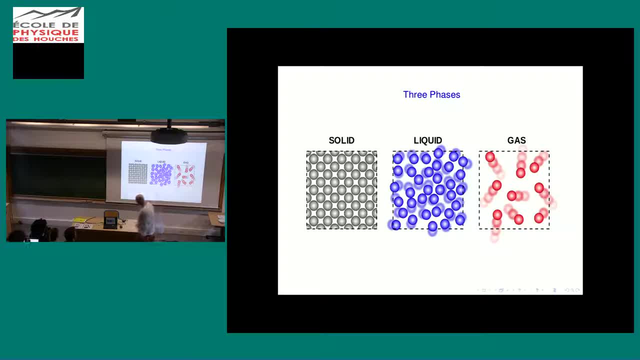 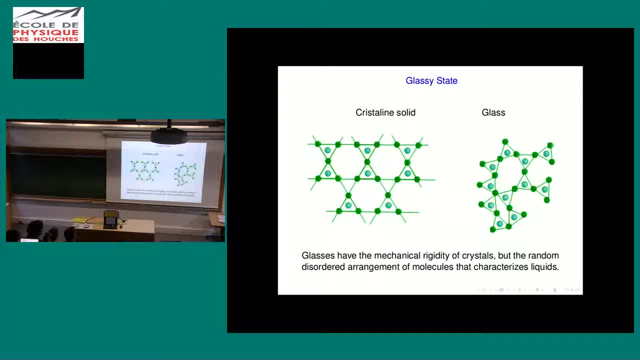 most of them do not have this ordered structure, but rather a disordered structure like a glass. So we have a glass here which is a solid but which has also a disordered structure, so it doesn't have a crystalline structure. 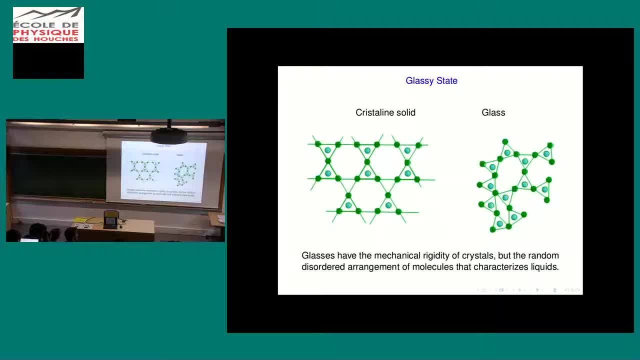 And it's more like a fluid with a very high viscosity. And so if a substance goes through a glass transition, what happens is just that its viscosity increases, and increases dramatically. So classical values are many orders of magnitude, So you have often 10 or 14 orders of magnitude. 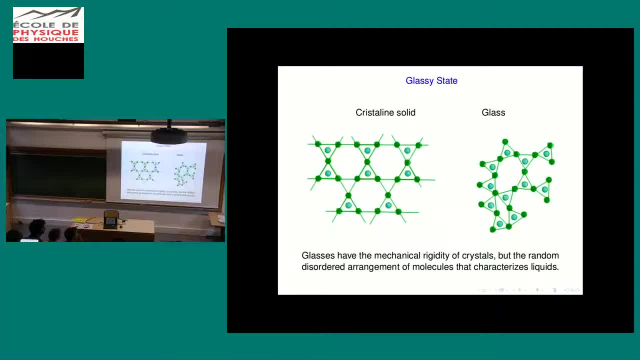 So the glass here is probably well, if you would wait for thousands of years it would probably flow down with time, but it takes a very, very long time. It has this solid aspect, but it has more the order of a glass. 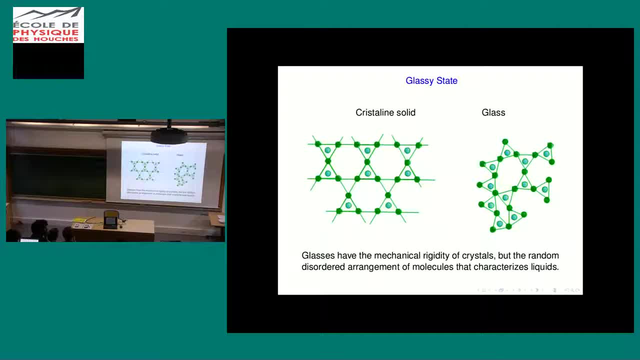 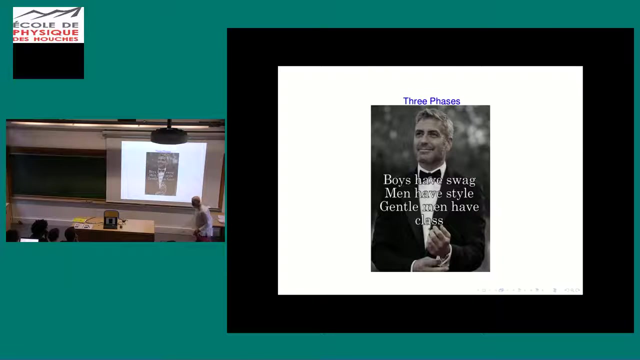 So I think- I'm not sure, of course- that the same thing happened in this air-sea interaction, and this is what I'm wanting to explore. So glass is the most interesting state when it comes to matter, but also when it comes to men. 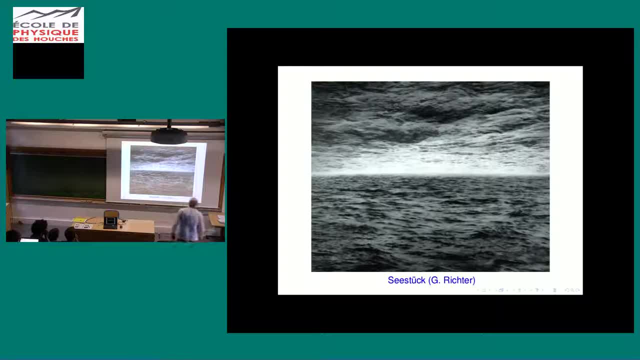 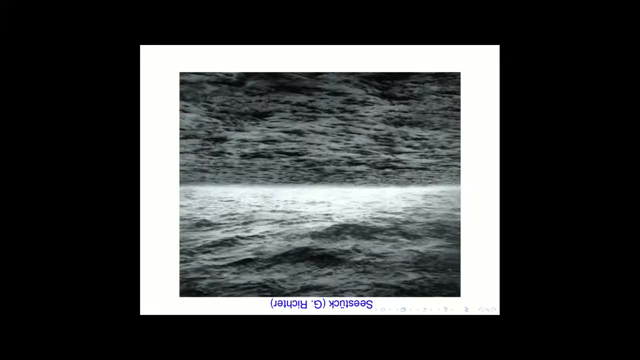 And so let me come back to this painting. And if you, when I hung up this painting in my office, I put it around this way, but I could have also put it around- I was hesitating. Maybe I should put it around the other way. 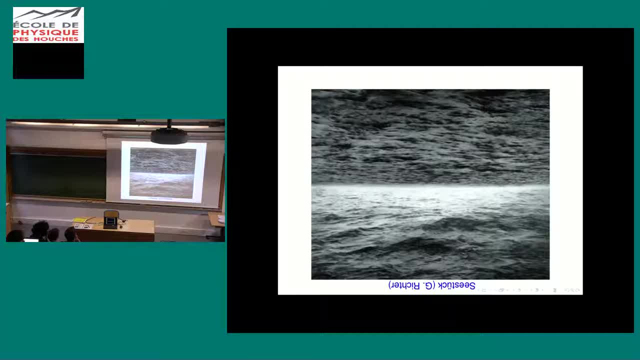 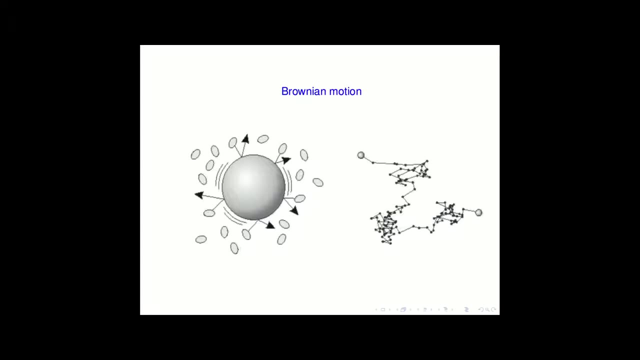 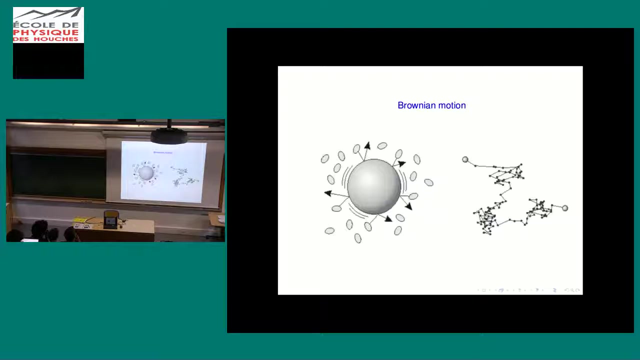 And so, after all, there doesn't seem to be too much difference between the atmosphere in the oceans and the view of this artist, And so this made me think about an analogy. This is the analogy of Brownian motion. So in Brownian motion, you have particles. 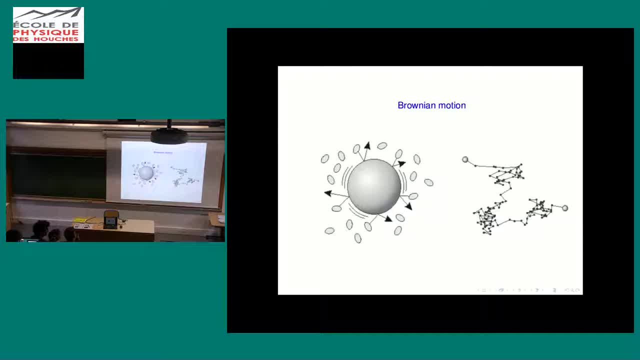 so big particles, which are sorry small particles, but big with respect to the surrounding molecules, And these big particles move around. I don't know if you have. I think everybody has heard about Brownian motion. I think it was in 1826,. 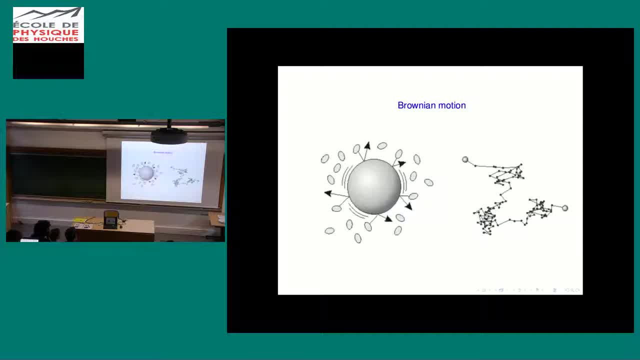 that this botanist, Mr Brown. he did some experiments. he had some pollen, he put it into water and he looked under his microscope and he saw that this pollen was moving around in a kind of a random way. And then he saw: well, this is. 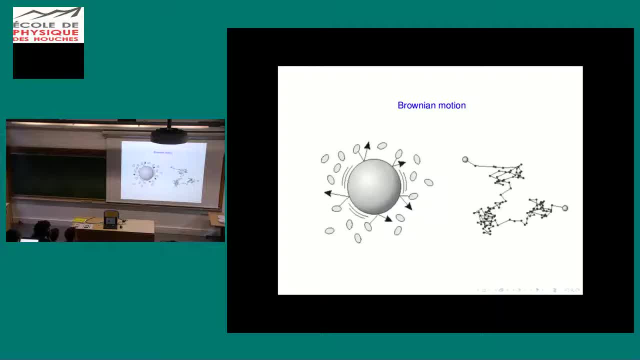 because the pollen is alive. he put some stone, he took some stone, he made some powder out of stone and did the same experiment, and still this powder was moving around and was what is now called performing Brownian motion. And so this is due to the atoms or molecules. 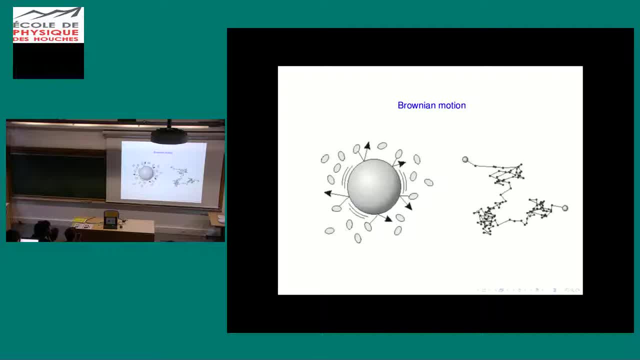 around this particle, which bang into this particle and drive it and make it go around. And if you look for a longer time then it does this movement like they are given here, so it moves in different direction, kind of impression that it moves randomly. 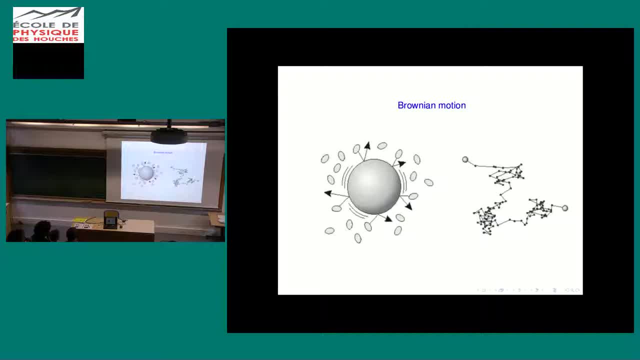 in different directions. So my idea, my idea was that the ocean and the atmosphere is a little bit the same thing, because you have the ocean, which is a lot of mass. above you have the atmosphere, which has a low mass. the atmosphere is moving very fast. 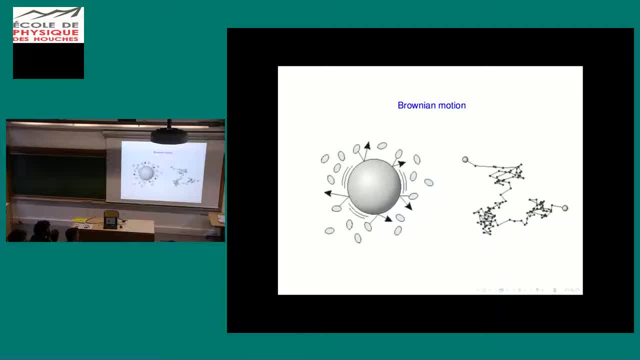 in all the directions, kind of a little bit randomly. it's turbulent and then it also pushes the ocean in different directions. so it's kind of an analogy to Brownian motion, And so I wanted to investigate if this analogy can be pushed even further. 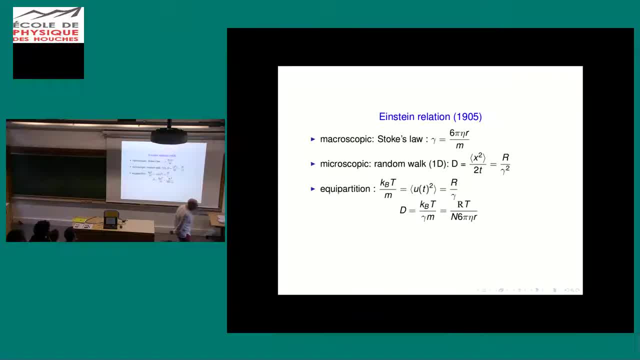 I don't know if people have talked about this or have thought about this analogy. I haven't heard about it. So for Brownian motion, it was Albert Einstein who solved the problem in 1905, so he published many very important papers. 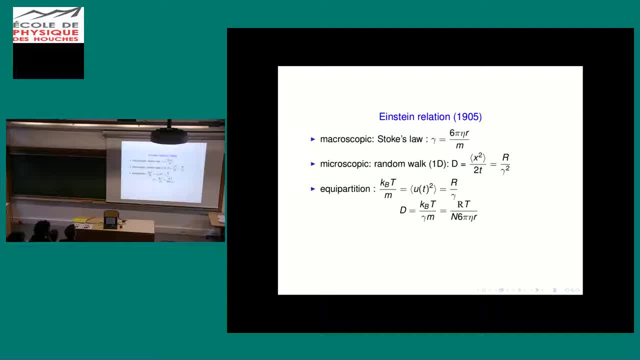 his most important. he published very important papers in 1905, and one of these his papers was on Brownian motion, and at that time it wasn't even sure that molecules or atoms existed. so kind of this work was also proof about the existence of molecules and atoms. 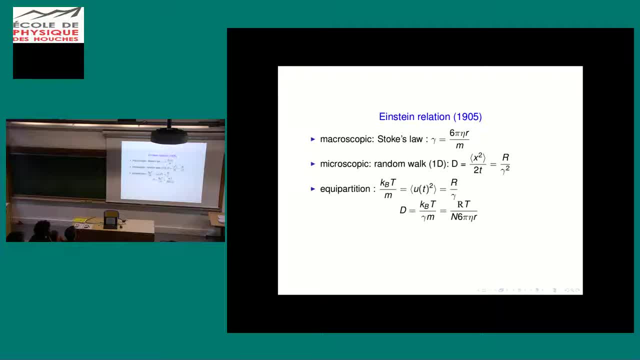 And so Einstein had the idea that actually the movement of this Brownian particle is governed by two processes. The first process is the Stokes force, so it's the force that is acting on any sphere which is moving slowly in a fluid. so if you have a viscous fluid, 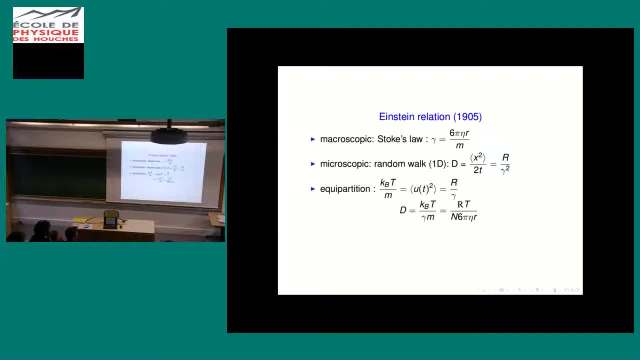 if a sphere is moving in, a viscous fluid, there is, and if it's laminar, then you can calculate the force. it's Mr Stokes who did it, and the inverse friction time is given by the parameter gamma, which is here. 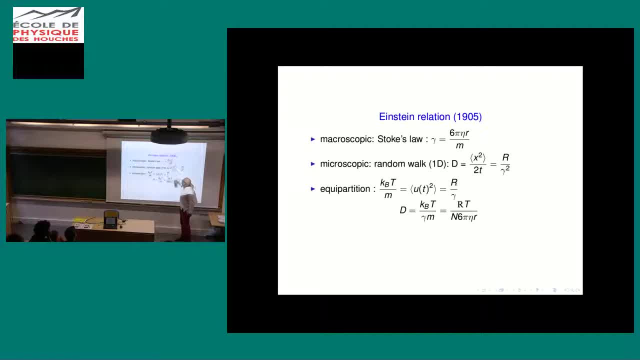 it depends on the radius and the dynamic viscosity Which are given here. so this is something which comes out of the macroscopic world. and then there's another thing which comes out of the microscopic world, which is the bouncing of these molecules, which is random. 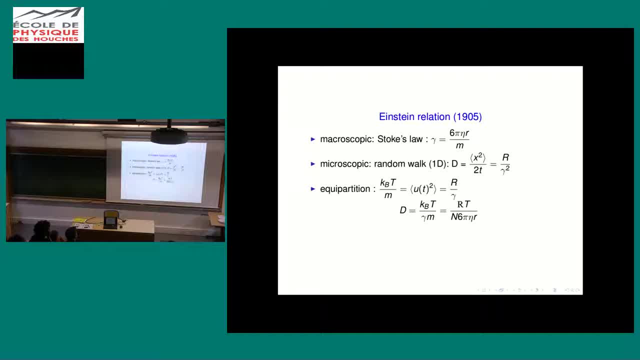 and the work of Albert Einstein was to find out that if you look at such a particle and you look at its distance, or more precisely at its square distance, how its square distance is evolving, and if you divide this by two times the time, then this is a constant D. 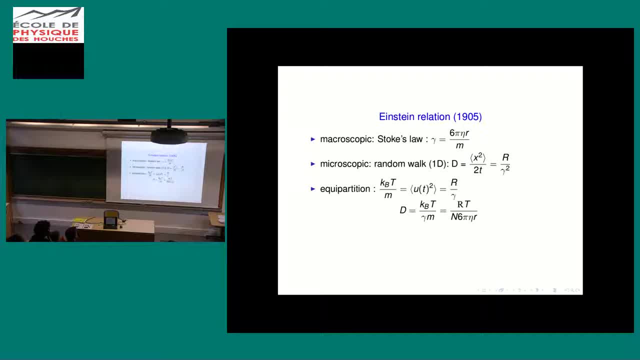 which is the diffusion constant. so he proved that this is the diffusion constant which you can potentially observe, and it's also equal to some R, where R is just the power of the kicking, of the forcing. you don't really need it here. 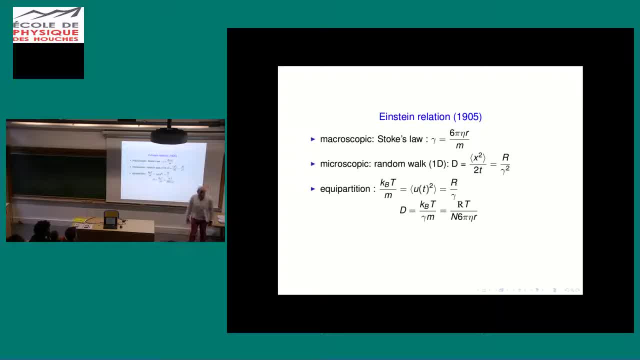 it just makes calculation easier. divided by gamma squared. Then Albert Einstein continued the calculations and found that the square velocity is equal to R over gamma. the averaged square velocity is R over gamma, and he also said so. this is from the microscopic world. 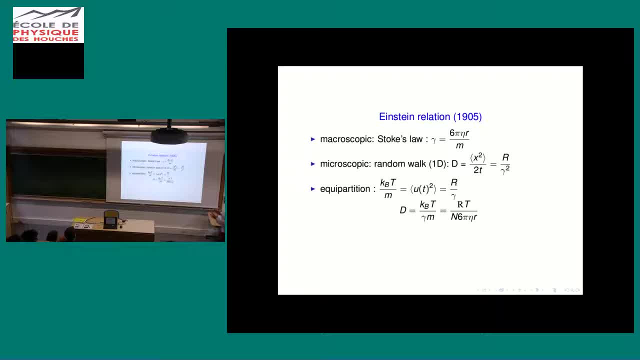 and from the microscopic world we also have that the equipartition of energies of every particle has the same energy, and so this Brownian particle has the same energy as a molecule, which is the temperature, or k Boltzmann times the temperature. 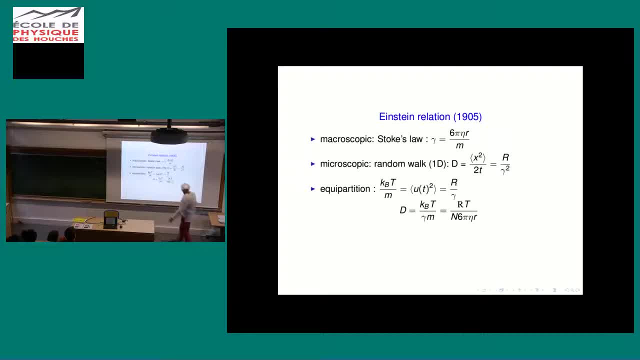 divided u squared is divided by the mass, and so if you put all this together and if you observe the diffusion coefficient, this is the gas constant, and then you can here. you have the Avogadro's number. so how many particles are in one mole? 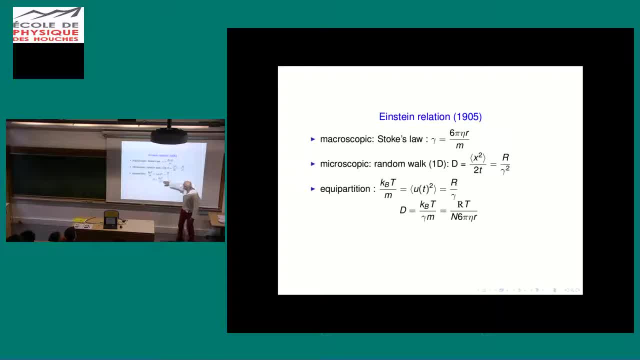 so if you can measure the diffusion coefficient and temperature, and if you know the radius, then you can actually obtain Avogadro's number. So these experiments were subsequently done by Jean Perrin, who then calculated Avogadro's number in many different ways. 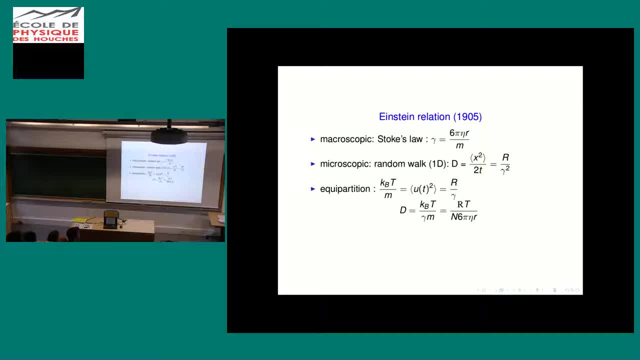 and they were all almost identical, and so Jean Perrin got the Nobel Prize for this work in 1926, Albert Einstein got it in 1921, Jean Perrin in 1926, and anybody knows what Jean Perrin did next. 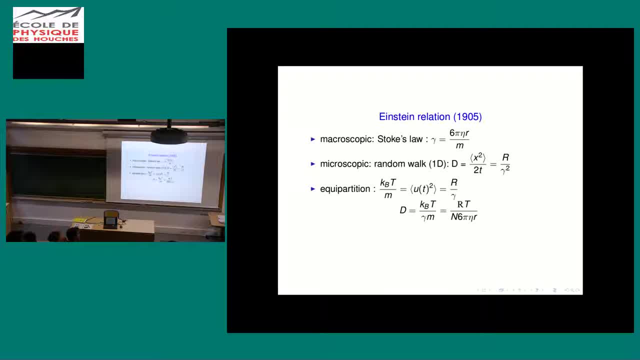 He founded the CNRS, so he's the founding president of the CNRS who's employing me and other colleagues here in the room. And so later on Langevin put up an equation which is called the Langevin equation, which is given here. 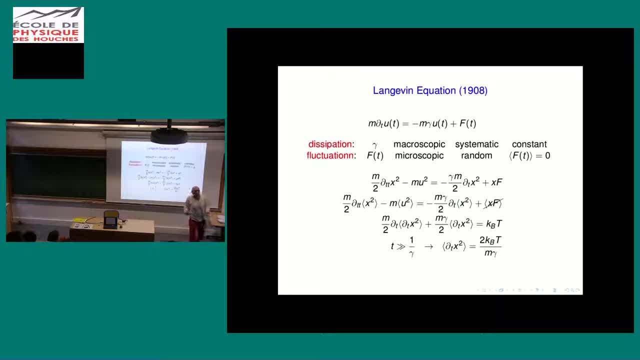 so most of you already know what I'm talking about. so if I have to go faster, don't hesitate. so I can also skip this, but I mean I need this for the sequel also. but so the Langevin equation is just: if you take the acceleration of the Brownian particle, 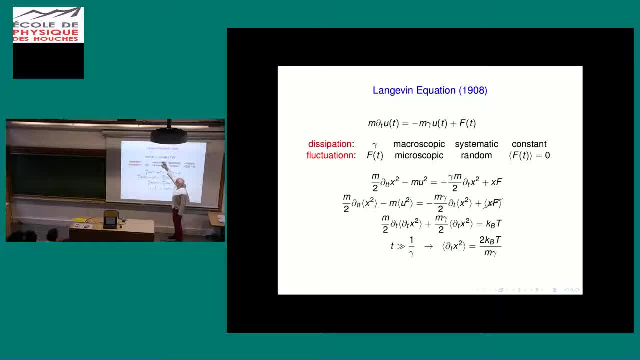 and it's subject to two forces: the Stokes force here and the kicking by these small molecules. and then, if you pose what I did here is if you say that well, u is just dtx, so I introduced x here. 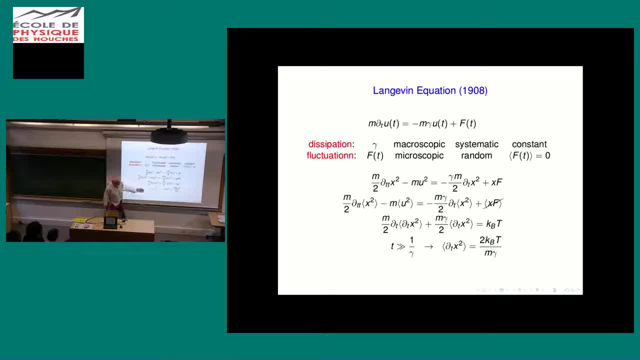 if you do some, just some basic calculation and you say that the force of the particles, the force kicking on the Brownian particle, does not depend on x, on the positions of the it's homogeneous, then you can drop this term. 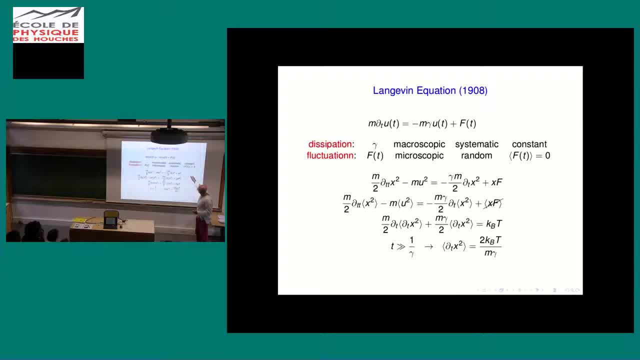 and then you get the same result of Albert Einstein in a few lines of calculation as it is done here, and so the problem with this equation was that at that time nobody really knew what f is. so this random noise, this, which is delta correlated in time. 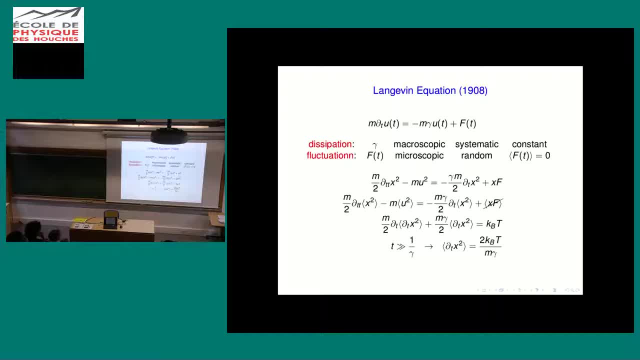 so, which has no correlation from one instant of time to the next. there was no mathematical theory about it. it took another 30 years for this theory to develop. it was done by Ito, and if you do this, Ito calculus. 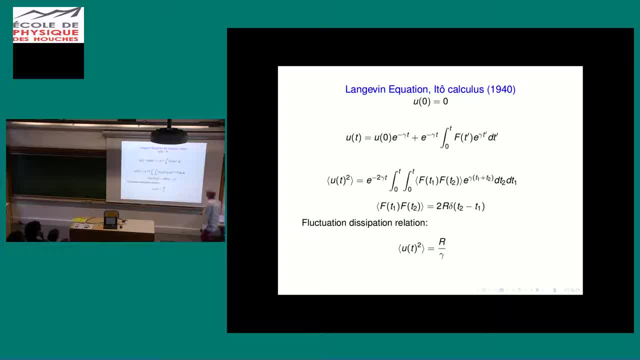 then you can just write the solutions very simply. so the velocity of the Brownian particle is just given by the initial velocity, times exponential function, times an integral over the forcing, because it's just a linear equation and you can also look at the square velocity. 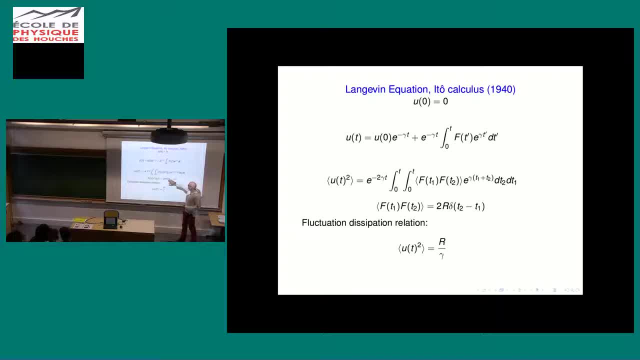 given here, and the square velocity is depending on the correlation. the average of the square velocity is depending on the correlation of the force and this is equal to this: 2r, where r is the strength of the forcing and is delta correlated in time. 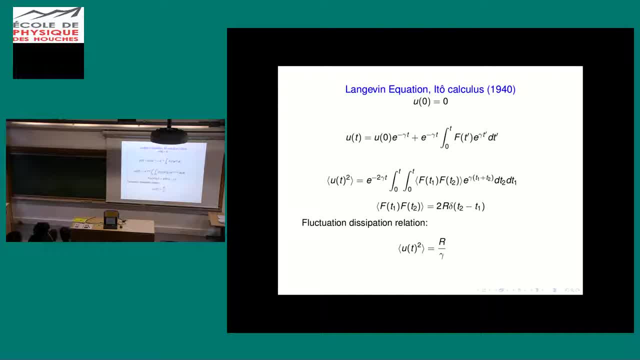 Sorry for the slide before this. is there an intuitive reason to understand why x and f should be uncorrelated? Because that's the main step. So actually this was already observed, apparently by Brown, that when he looked at two particles who were moving around, 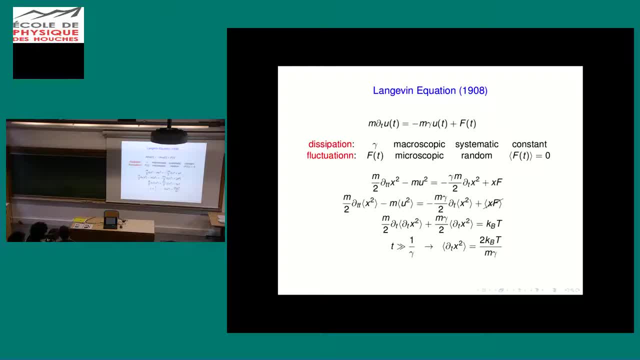 even if they were a very small distance, they were moving independently. So this particle moving here, Brownian particle moving here and Brownian particle moving here didn't have any correlation. So, And what you have here now is you get an equation again for u squared here. 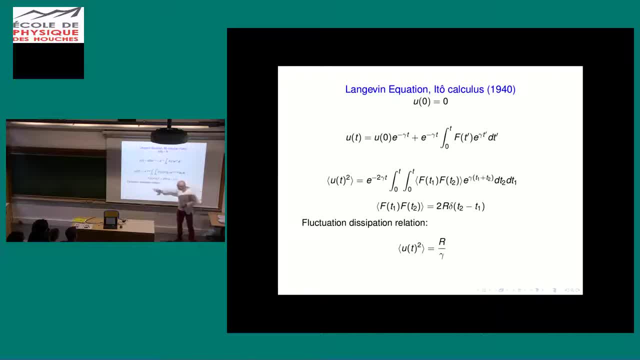 which is equal to which is given by equipartition of energy and what you see, it connects the forcing and the dissipation, So it connects the microscopic world and the macroscopic world, And this is known as the fluctuation-dissipation relation. 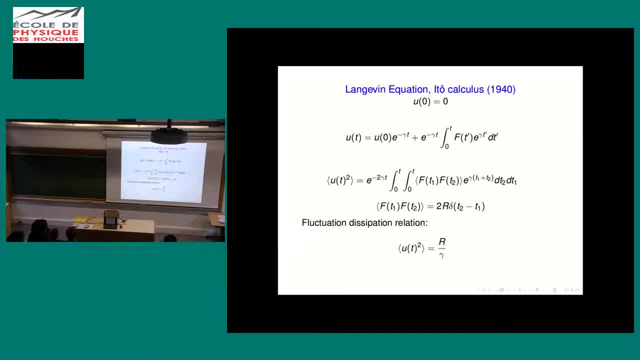 So at some point we can see that it's not much of a surprise, because the dissipation and the fluctuation, they come from the same origin, from the fluid around. So somehow they should be connected And establishing a connection between, let's say, the kicking of the system. 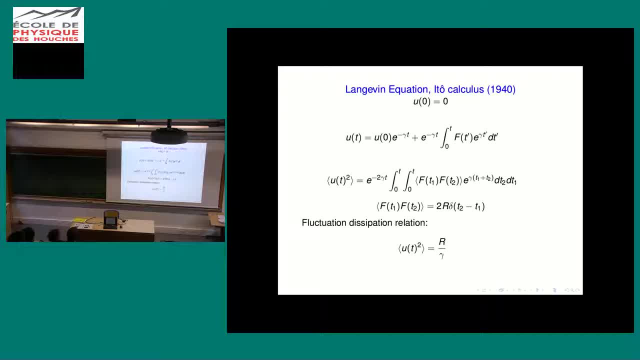 and the dissipation of the system is given by this fluctuation-dissipation relation, And for the Brownian particle it's just done by the equipartition of energy. So we know this, then we know the relation between these two. 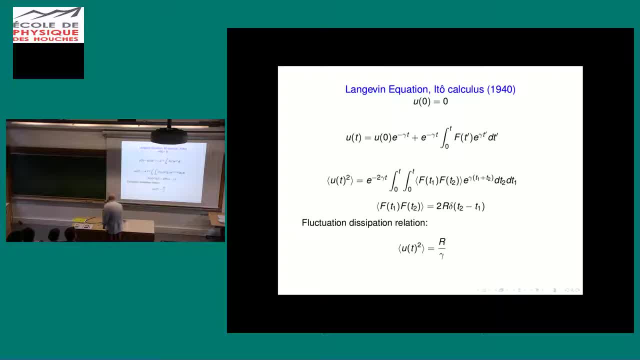 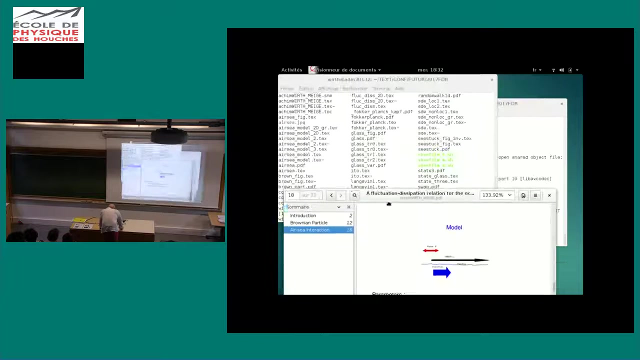 So this was the little excursion to Brownian motion Before I now go on with my model, And this is the same picture that I have shown before, And so now I'd like to show you a film about what's happening, And so I made numerical simulation. 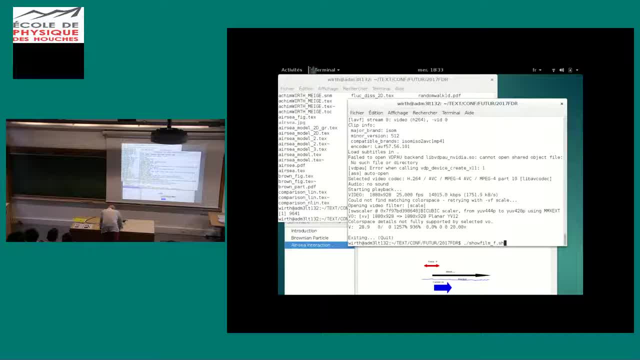 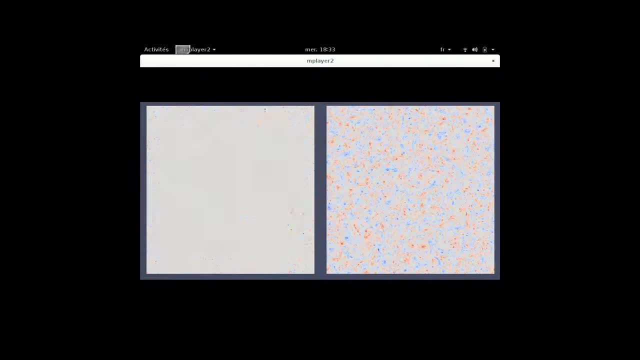 of this problem And this is what you see here. So, as you can imagine, left side is the atmosphere, right side is the ocean, And the atmosphere is forced again by the same type of forcing. So at every instant of time, the vorticity is projected on a mode. 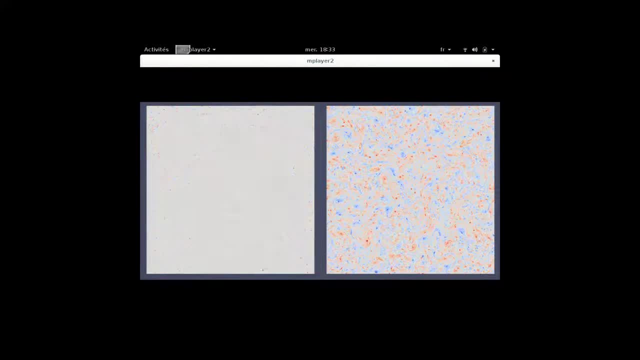 which is the mode k, equals 80 here. So you have 80 maxima and minima in this line, and it's kx in this direction Which gives the forcing, which is restored always to its initial value, And only this mode is kept fixed. 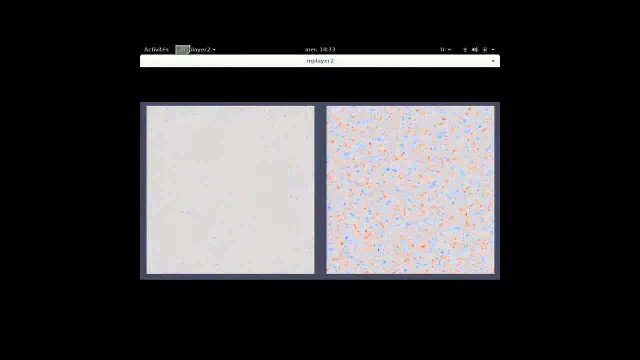 and the other modes are not touched upon And what you see is now the atmosphere moving around And actually the ocean you almost don't see moving. So I have a film which moves a little bit. So the same film, I can make it move a little bit faster. 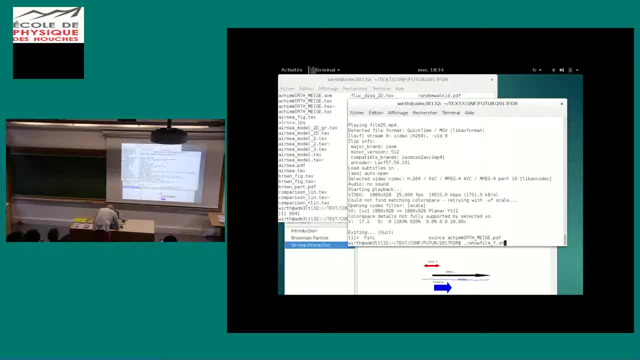 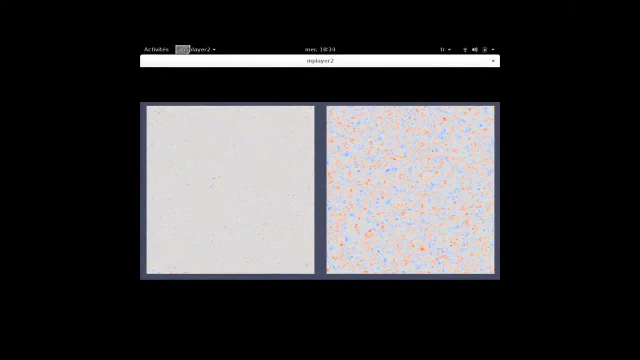 So this was slower. This was already the fast version. So the problem with it is that I had a slow and a fast version, but my small computer- here the fast version- goes very slow because the computer is too the graphics card is too small. 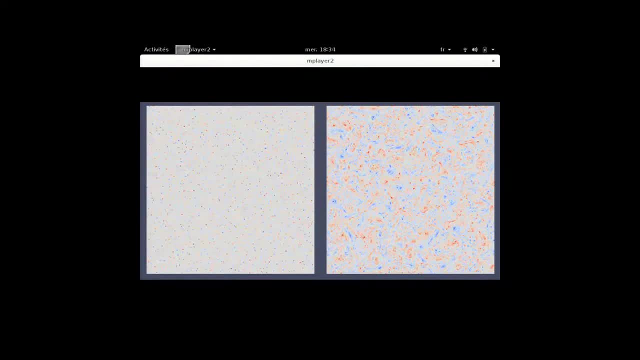 Anyway, when I show the slow and the fast version, on the slow version you only see the atmosphere moving. On the fast version you see the ocean moving, but the atmosphere is very. I mean, you don't really see movement because everything goes so quickly. 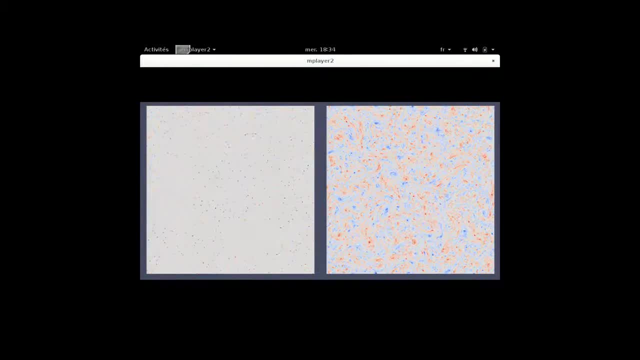 So this is the problem in air-sea interaction: that you have an atmosphere which moves very fast and you have an ocean which is moving very slowly, So you have what's called a stiffness problem, And usually this is done by to facilitate the integration. 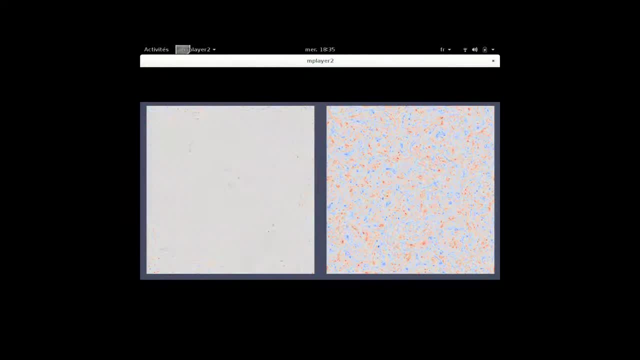 the ocean and the atmosphere are integrated on different resolutions in time and space, And that's not what I do. So I integrate the ocean and the atmosphere at the same grid points with the same resolution in space, same grid points and also the same temporal evolution. 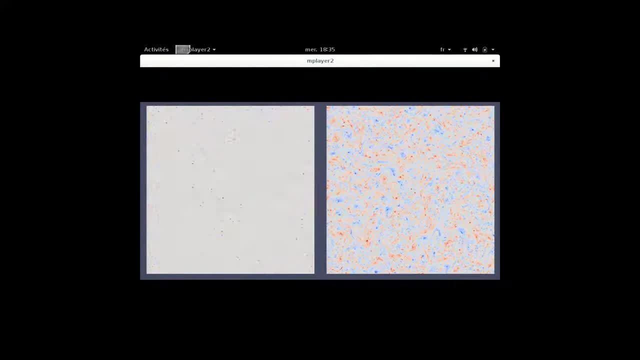 and the resolution, and there is an exchange of of information at every, at every time step. So I've really a system is two parts, a fast part and a slow part, and they involve, evolve together, And this simulation has a resolution. 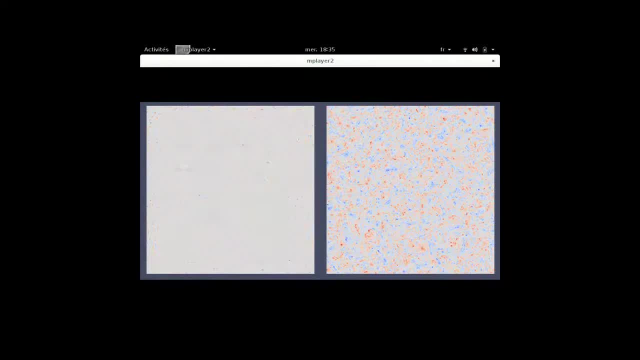 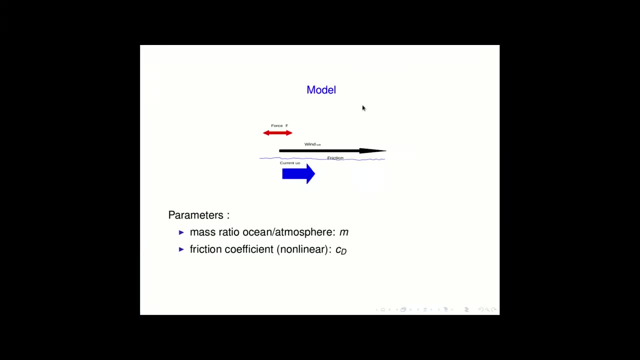 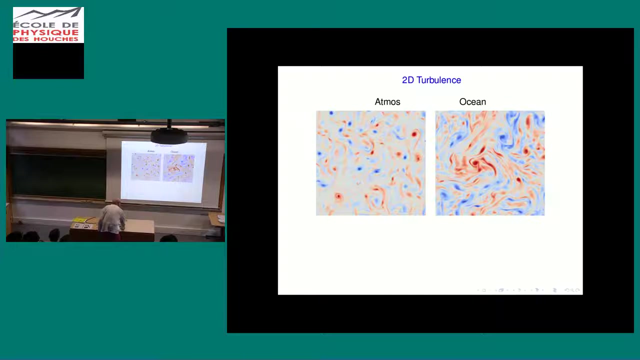 spatial resolution of 4096 square points. And so let me go back to my presentation, And so here I again have a picture of of of this, of the atmosphere in the ocean. Here I just made a zoom. 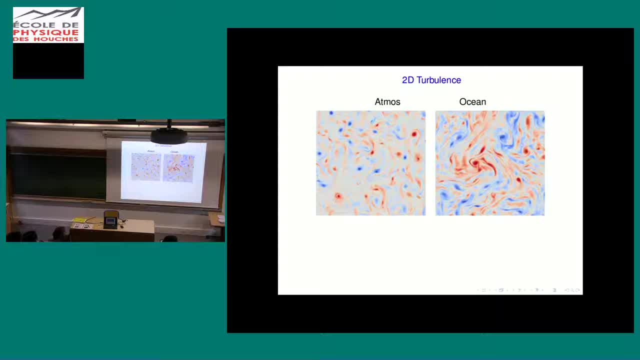 You just see one hundredths of the domain which I integrated just to to show you that this small eddies which you just saw a a moving around, They're really resolved and you see in between them, in the atmosphere, a lot of filaments. 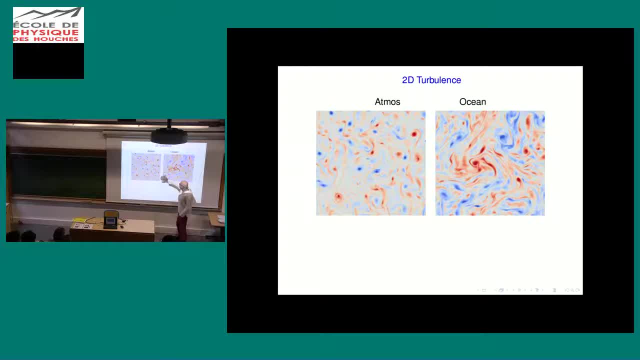 So a lot of filaments and because the resolution is very high, I resolve all this. dynamics, The dynamics in the ocean looks also this large eddies and very, even more seems to be even more filaments in the ocean. So my question is: 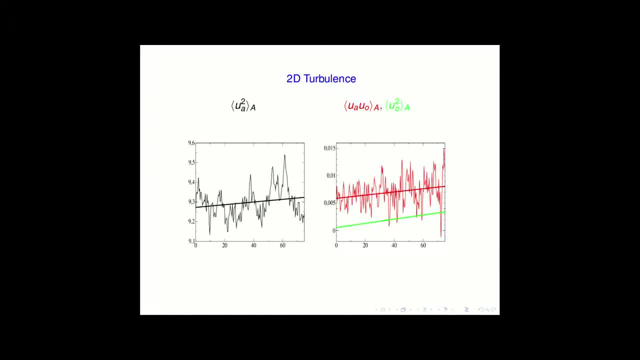 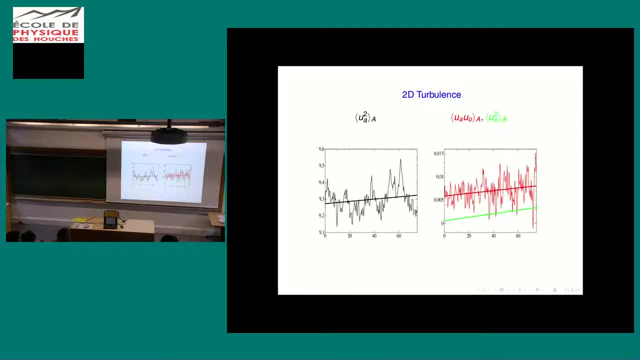 I wanted to analyze it a little bit more, more quantitatively, and to this end, I do the same thing what we did in Brownian motion, or what was done in Brownian motion: I looked at square, at the square velocity, If you see. 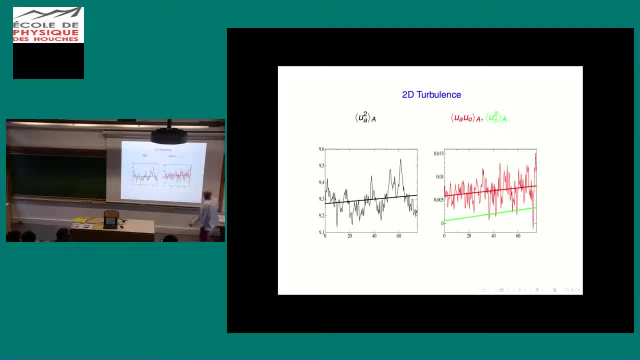 look at the square velocity in the atmosphere. you see the zigzag motion here and this is the best fit of a straight regression line. I did the same thing for the ocean. Ocean actually don't see much zigzagging, because it's it's hidden behind the 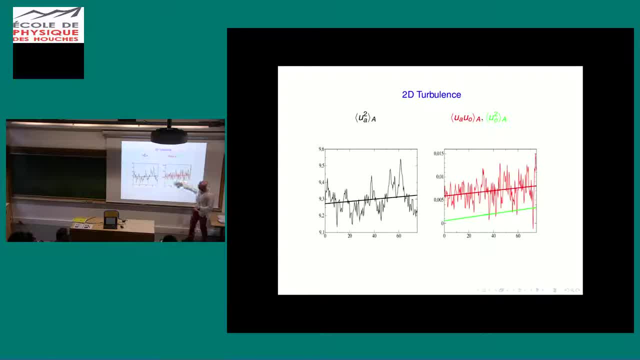 the best fit line. So the ocean is evolving almost on a straight line And I also looked at the at the correlation of the atmospheric and the ocean, atmospheric and ocean velocities, which is this red line, and the best fit is this red line. 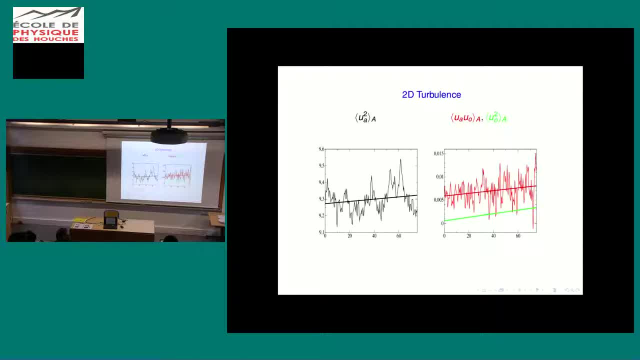 And if you look at it, it seems that they're both kind of parallel, right? I mean, they're not very far from parallel. So how can we understand this? To understand this, well, I started with the most easiest model you can imagine. 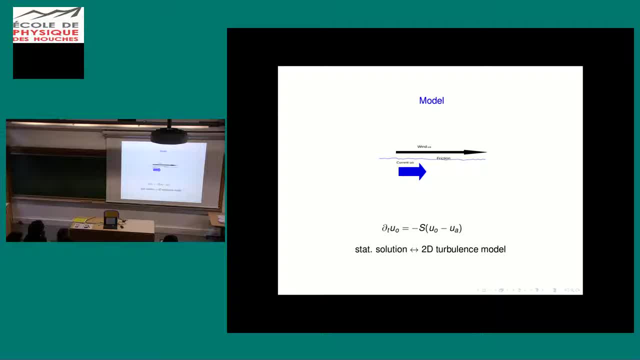 which is this here. So now I'm going to talk about local models, So zero dimensional models. So I'm I'm neglecting the horizontal exchange of momentum and now everything is zero d. So I have one variable for the ocean, I have one variable for the atmosphere. 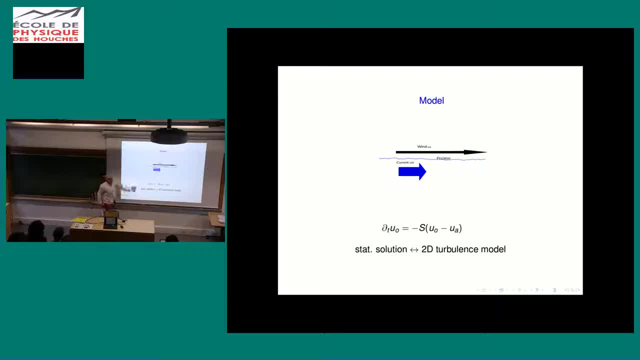 and they interact and the ocean velocity is zero And the atmospheric velocity is uo and the atmospheric velocity is ua And I have the acceleration of uo is given by stability parameter s times this. So here for a short moment, I do not have a quadratic drag. 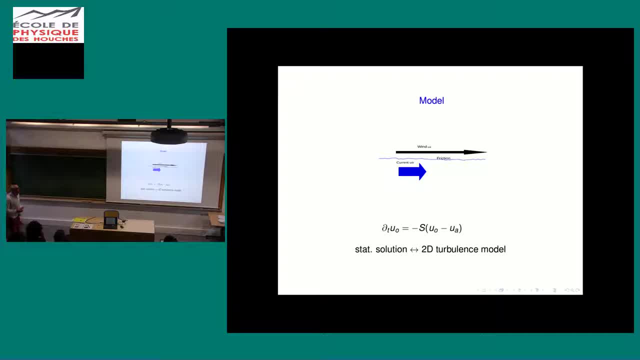 I have linear drag now. I'll come to quadratic drag later And if you look at this equation, it looks like, I mean, it is a Langevin equation. You have the atmosphere here which is moving very fast, And you have the ocean here. 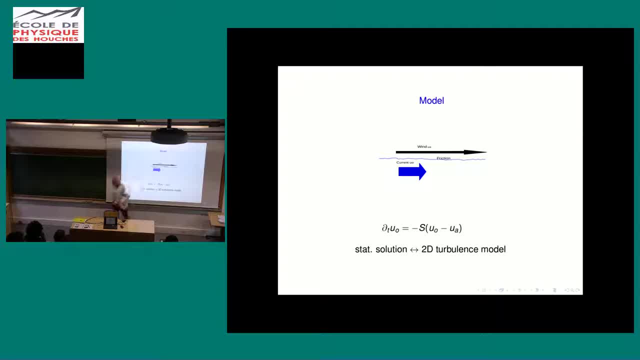 which actually dissipates. And if you, if you multiply this equation by uo, what you get is uo dt. uo is equal to minus s uo squared minus ua uo, And this is actually one half uo squared. 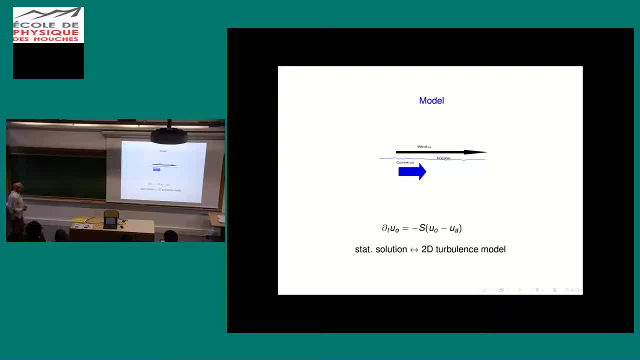 And so the energy, the energy input, the energy increased in the ocean is a function of the difference between uo squared and the correlation between the atmospheric velocity and the oceanic velocity in this very simple, in this very simple model, And so it's a Langevin equation. 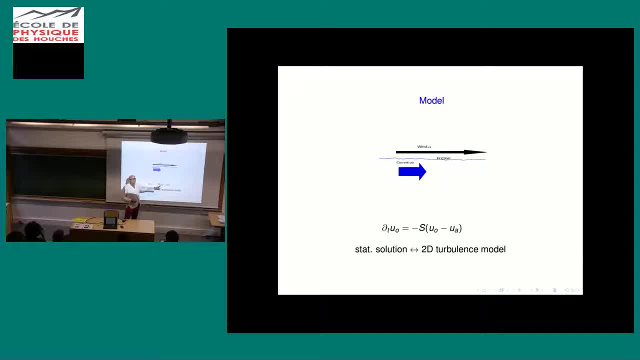 Here where? here you have the systematic, the systematic drag, And here you have the agitation by the, the atmosphere. So it's the same same thing. However, this model is not good. It doesn't work because it will. it will go to a stationary state. 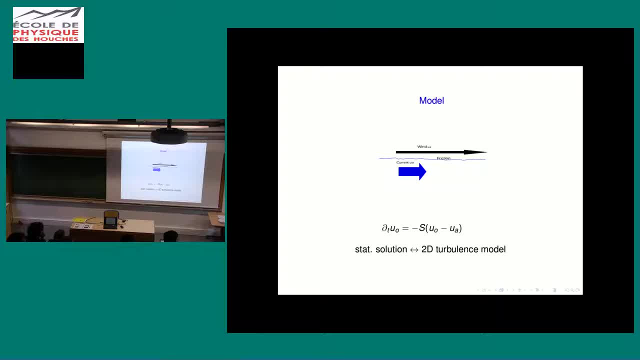 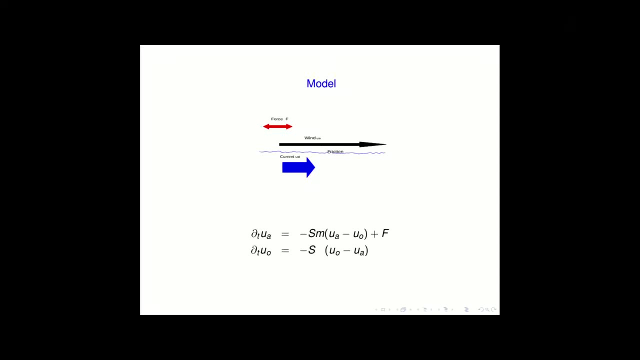 And in my simulations I didn't find a stationary state, But it had this linear increase of all the square quantities. So I had to go a little bit further, make the model a little bit more complex, And what I did is I just 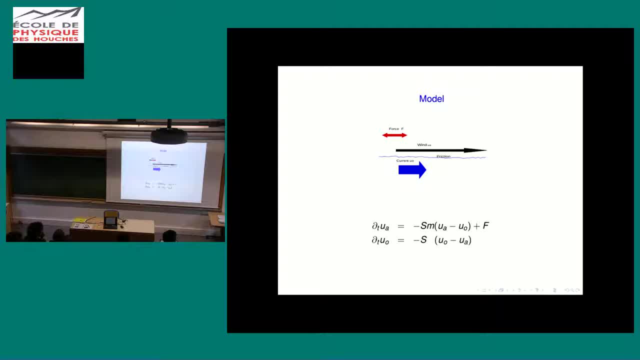 integrated, added a variable for the atmospheric, a dynamic variable for the atmospheric velocity which is given here. So now I have a forcing which is applied to the atmosphere, which evolves and which then acts on the ocean. And if you look at this equation, 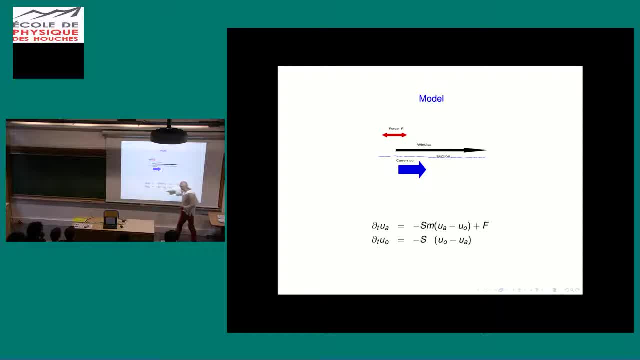 you again have this Langevin equation which is applied to the ocean, But you have a different equation for the atmosphere. This is the atmosphere itself, which appears here, is also subject to this friction, And you have a forcing which is applied here too. 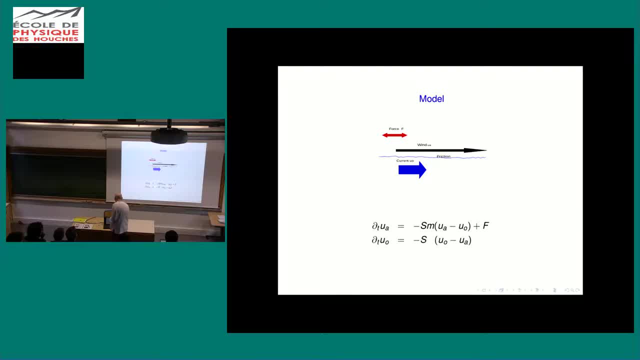 So it's a little bit more complicated, but not much, because it's still linear equations And actually what you can do is you can find, you can, you can have a shear mode. So U? S is just this shear mode here And you can have a total. 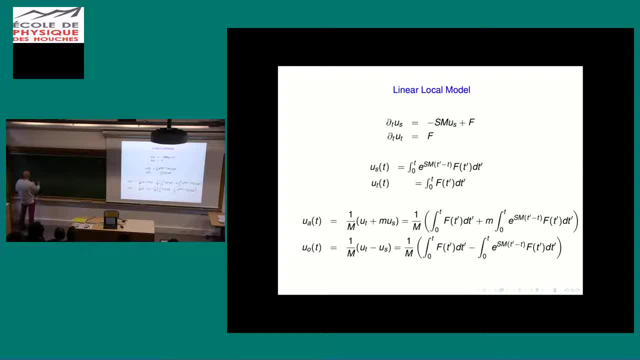 a total inertia, which is U A plus M times U O. where M is this 100? because the ocean has a mass which is 100 times larger than the atmosphere. And then I have another variable which I haven't written, So M is equal to. 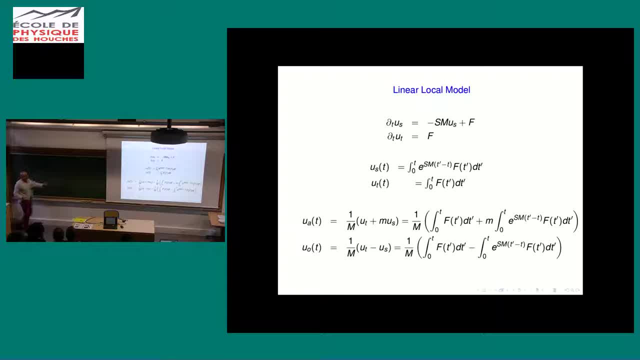 capital. M is just M plus one, So it's actually the total mass, the mass of the ocean, which is 100, plus the mass of the atmosphere, which is equal to one. And so then you have, if you, if you write down this equation, 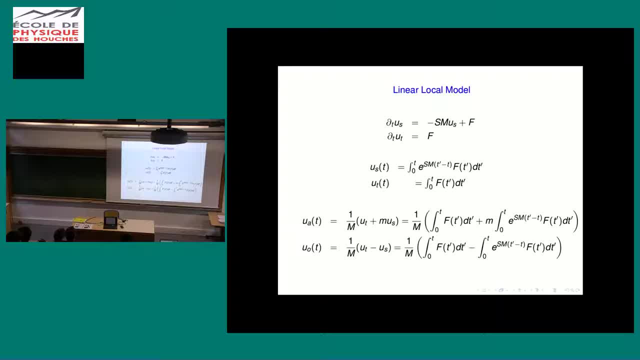 equations. then it becomes very easy because actually you have a Langevin equation for the shear mode and you have a random walk for the total, for the total inertia mode. So you have the two modes which are completely uncoupled And one is just the total inertia. 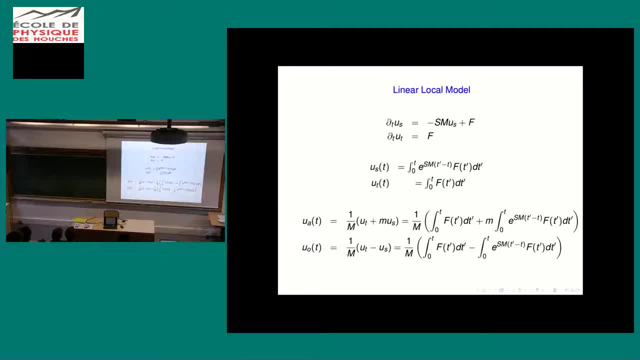 and one is just the shear mode, And of course these are linear equations. You can solve for U S, U T, and then you just put this into the equation, You inverse this and then you put this for U A and U O, And what you get is just these integrals. 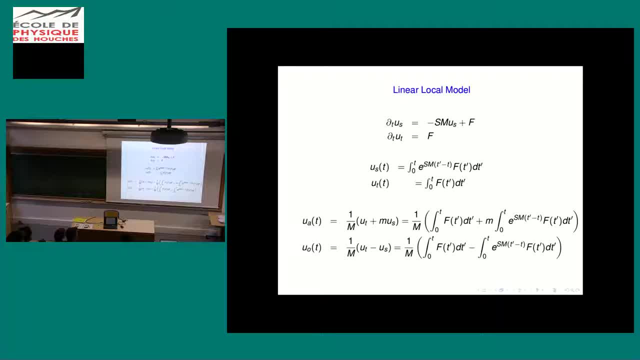 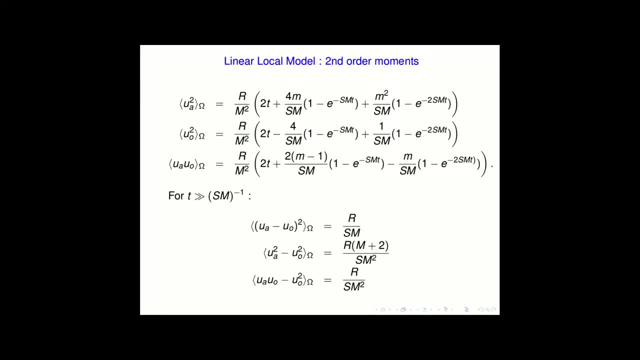 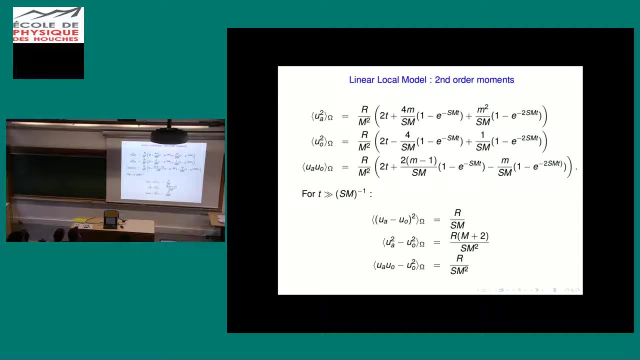 which are just linear equation integrals. And this is what you get from this. And if you look at the square quantities, you just do the calculation, You look at the square quantities and then you look at averages. So the averages of the unsquared quantities are zero. 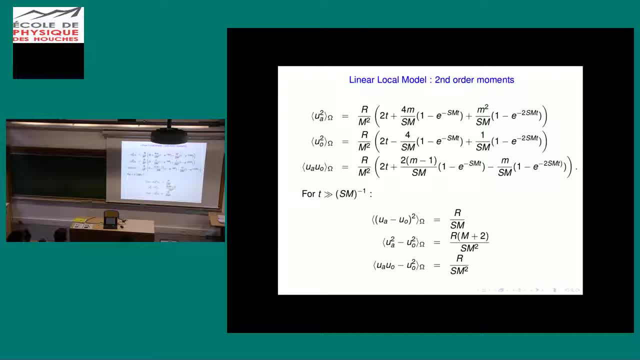 I mean, the first thing is zero, so it's just, everything is zero. However, the square quantities are not zero And if you do the calculation, you just find what's given here, So you have a linear growth in the ocean. 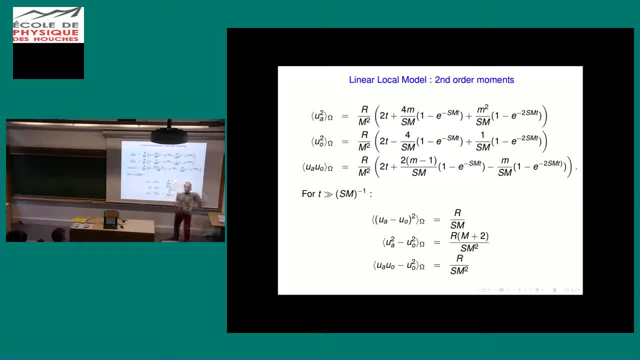 in the atmosphere, the ocean and the correlation between the ocean and the atmosphere. You have this two T here which comes from the random walk. So the random walk is like the second order moment is increasing linearly in time And then you have other terms. 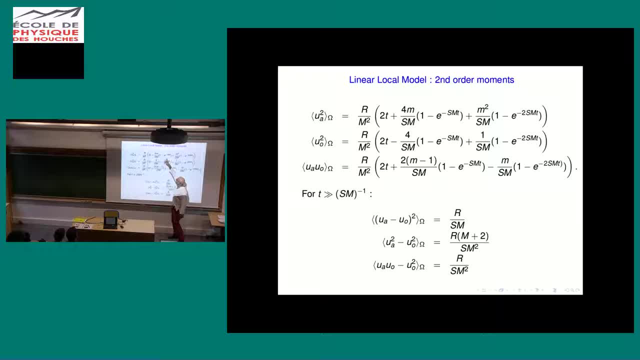 And so if you look for a larger time, so if you forget about the initial part, then all the exponentials here are zero. And if you look at differences of these variables, so U A minus U O squared, or U A squared minus U O squared. 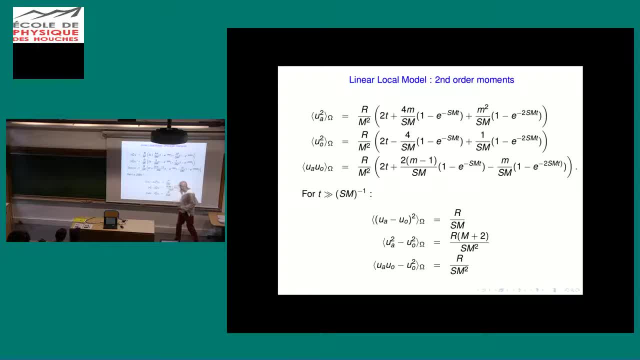 or U A, O, U O minus U O squared, then this linear term drops out, because it's the same in all this, It's always two T And you get this just the results, I mean just the calculations. Okay, very good. 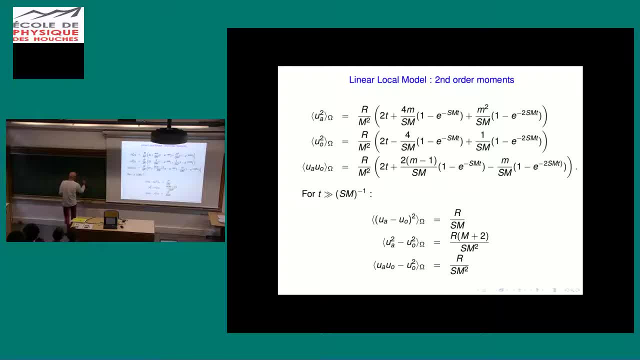 So S is the friction coefficient, M is 101.. So it's just the mass of the ocean per unit area, as compared to the mass of the atmosphere, which is one. So this is 100, so it's 101.. And R is just the strength of the forcing. 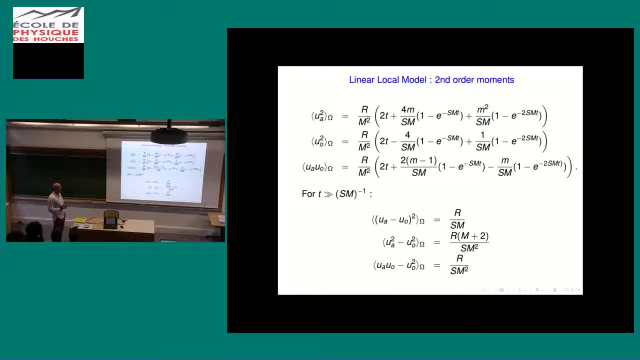 So how strong I'm kicking the system. Yes, Yes, So Hasselmann started to introduce- I think it's him who started to introduce this method into climate science, but he looked only at heat flux, So he was on heat flux. 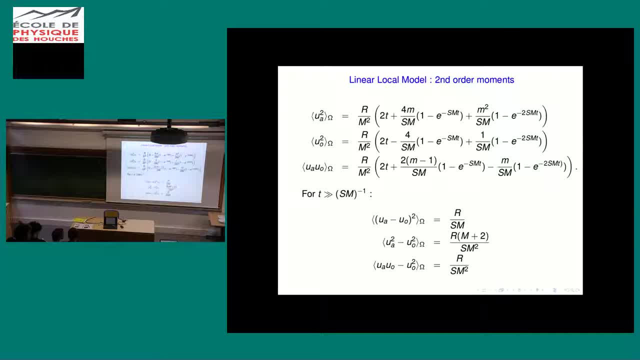 I think, and he didn't do these calculations, I guess He did Fokker-Planck equations but he didn't do the statistic differential equations and it's somehow the same and I think the same things can actually be done on heat flux. 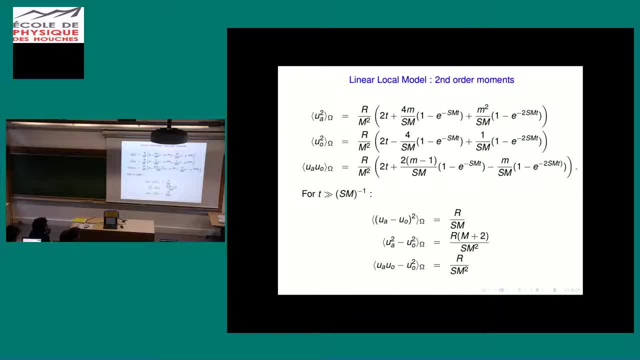 I mean I think it should be kind of identical, because the heat capacity of the ocean is much larger than the heat capacity of the atmosphere and should be a little bit the same things happening. So Hasselmann did this and Franklin Yule and Hasselmann in the 70s, I guess somewhere. 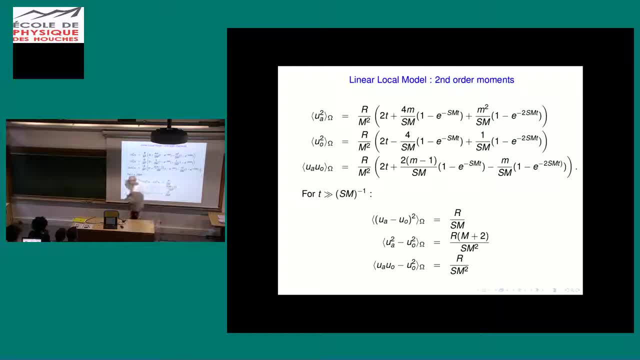 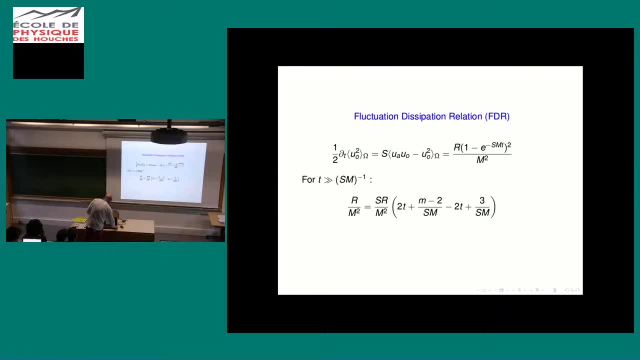 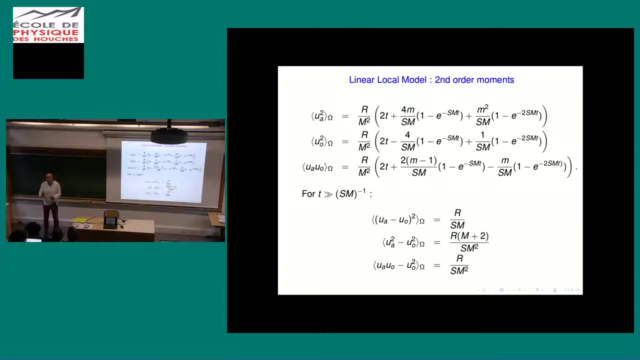 around this dates did similar things, similar things. So yes, so next slide. yeah, No Coriolis force. Oh yeah, I should have said this. There is Another question. At the moment, there is no Coriolis force. 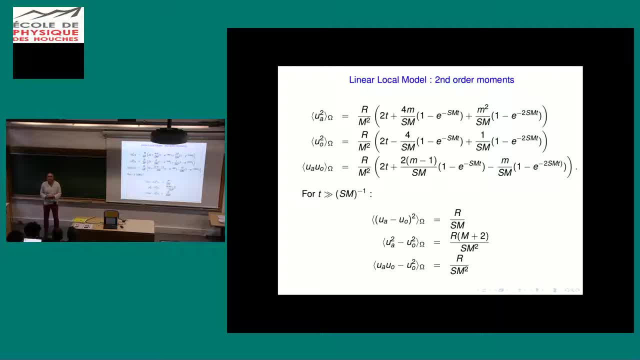 Okay, but in the previous slides, in your previous work, you included Coriolis force in your. So in the work at the past I included Coriolis force, and the Coriolis force I think is very important for the glass transition because it introduces me to scales, because you have 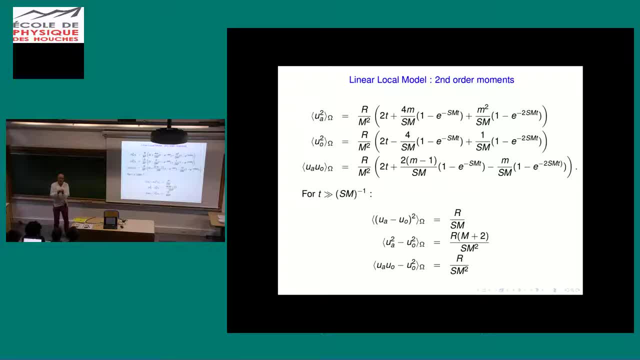 a Rossby radius of deformation for the atmosphere And the ocean. so you have two characteristics scales in the system and this is often thought in condensed matter. it's put forward that this is very important for glass transitions, that you have two types of length scales or two types of molecules which interact, which 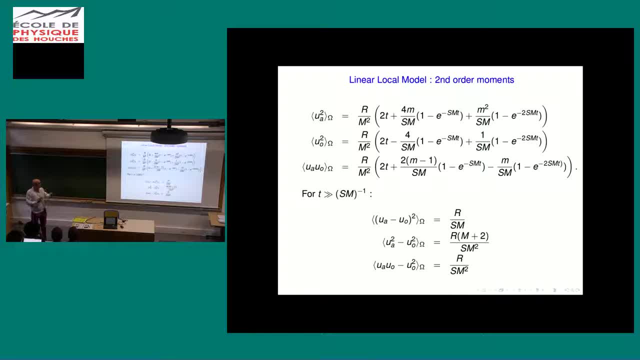 are different, but not too different, And so here, for the moment I don't have it. but the next step is very important to include to do the same things on the F-plane. Okay, But for the moment it's not on the F-plane, it's two-dimensional turbulence. 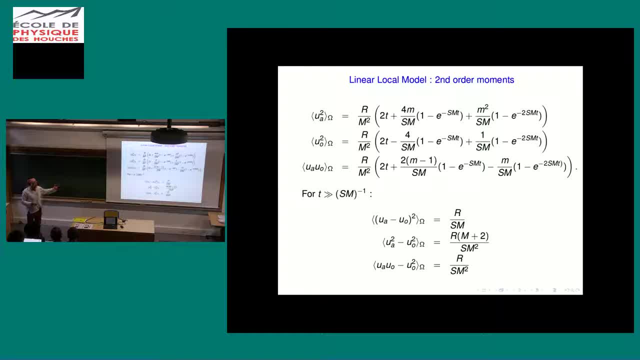 Okay, But I mean, technically, changing the code into a quasi-geostrophic code is something which is done in two hours. I mean it's not, There's no technical problem with it. Okay, And also previously, if you included Coriolis force, the deformation radius between atmosphere. 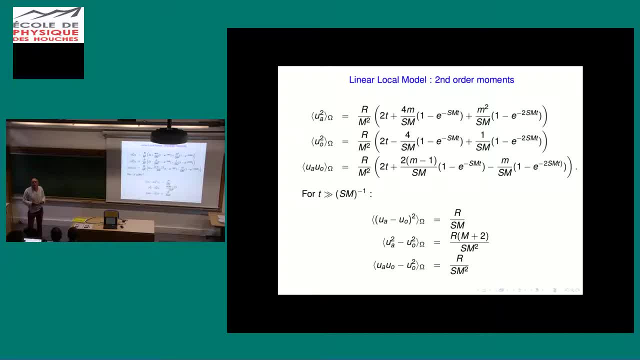 and ocean is very big, so you resolve both of the deformation radiuses. Okay, Yeah, so that's why in the previous I had 2,000 grid points also, so I resolved the 20 kilometers of the ocean and the 200 kilometers of the atmosphere. 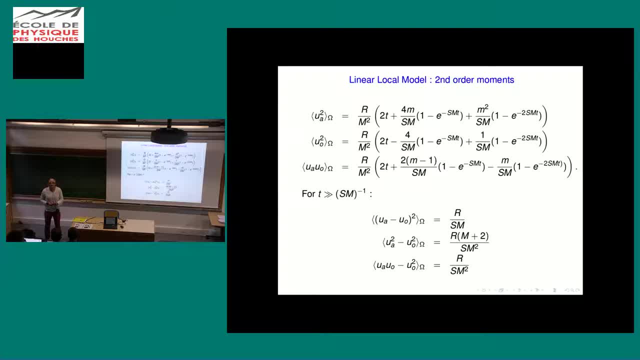 So the computation is quite expensive. It was an expensive calculation and this is why I stopped using shallow water, because with shallow water it was too expensive. I couldn't push it further and this is why now I do. two-dimensional turbulence and 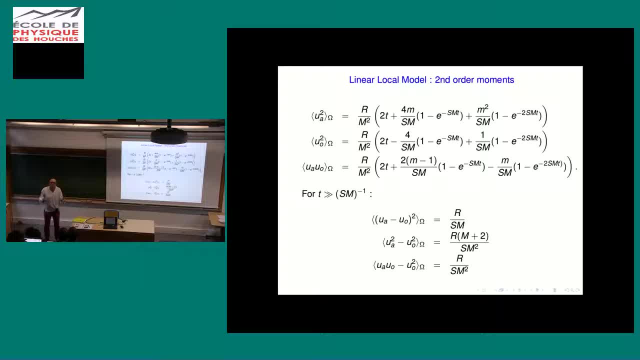 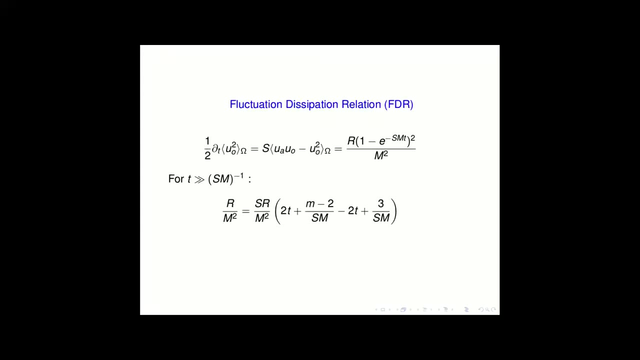 later on quasi-geostrophic, Because it's much cheaper numerically to integrate these equations. That's a very good question, thank you, Okay, so if you now write this equation- this which is written on the blackboard here, 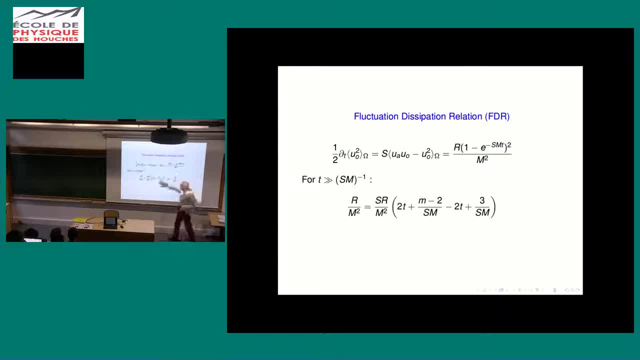 if you write it again here, then you see that for long times you have, on the left side, r over m squared, And then on the Then this side, This, this term here is what's given here. so this is the correlation of the atmospheric. 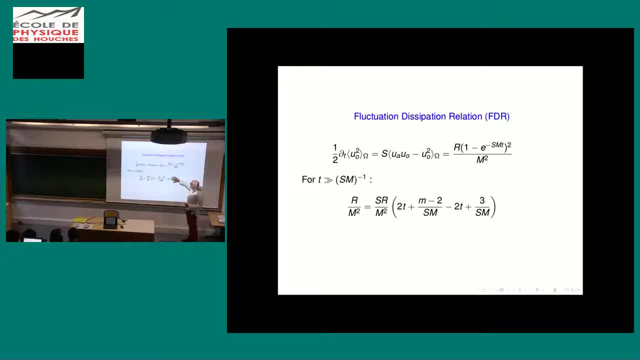 velocity and the ocean velocity and the autocorrelation of the ocean velocity is this, And this is kind of the equivalent to the fluctuation-dissipation relation which is given, in which is given, in which was calculated for the Brownian motion here. 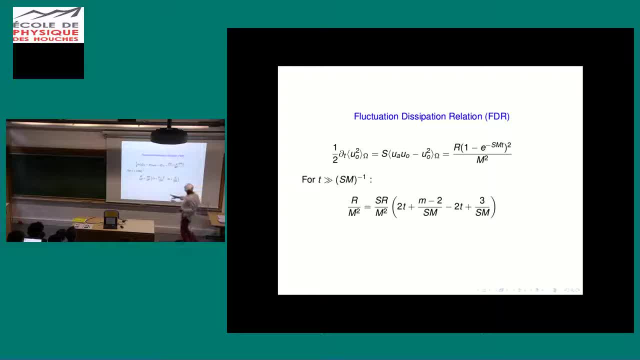 I calculated it, or I showed it, because it's not really a calculation, because it's just made. This is equal to this, but I mean it's trivial, it's tautological, but it says how this, The two, the two terms or the three terms combine to each other, and it really works. 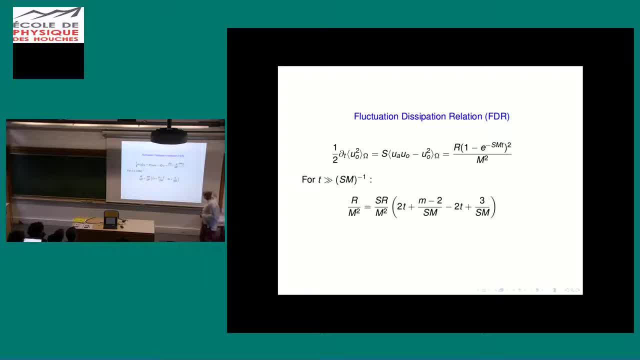 out that you have this, this relation between the increase of the variance of the ocean square velocity and the correlation between the atmospheric and the oceanic velocity and the oceanic velocity squared. So This is kind of the fluctuation-dissipation relation, and then, well, this was the linear. 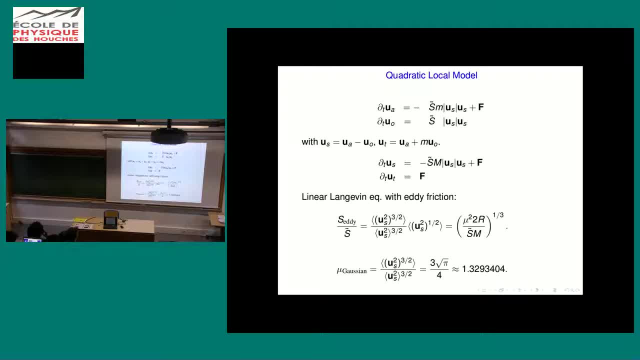 model. but friction is not linear at the surface or between the ocean and the atmosphere. So at one point I went to the quadratic model. So the quadratic model is given here. so it's still zero-dimensional. I don't have anything, it's just zero-dimensional. so U. 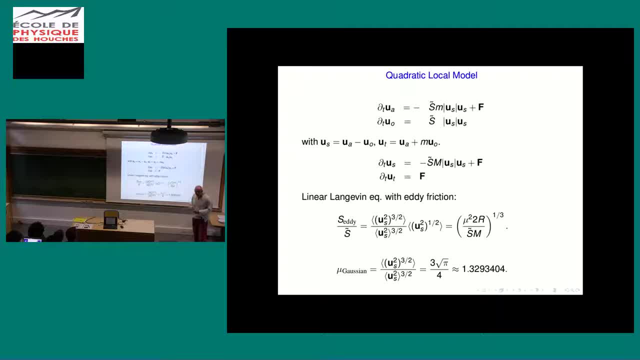 But now we have vectors. Before I just wrote scalars, because in the linear model what happened in the x-direction is independent from what happened in the y-direction. This is no longer the case if you have quadratic model, because now the U component depends. 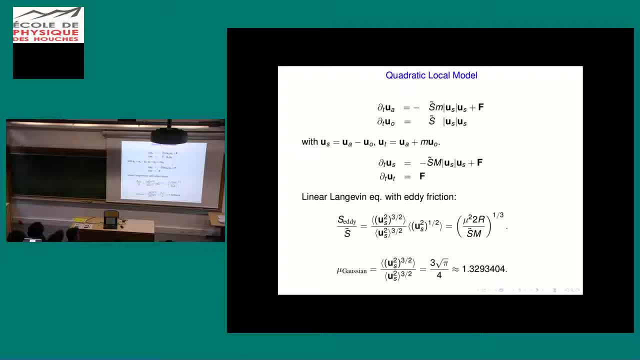 also on the V component. the V component depends on the U component, So you have to use vector notation, but the rest is the same and you have. The new thing is, of course, that you have this absolute value of the shear. 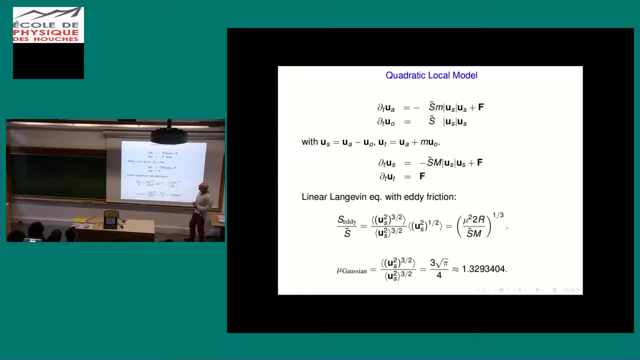 Okay, The shear velocity, as is already written on the blackboard, but you can still separate in a shear mode and a total mode. and then what I wanted to do is I wanted to see if I can reduce this a little bit more complex model on the simpler model to the simpler. 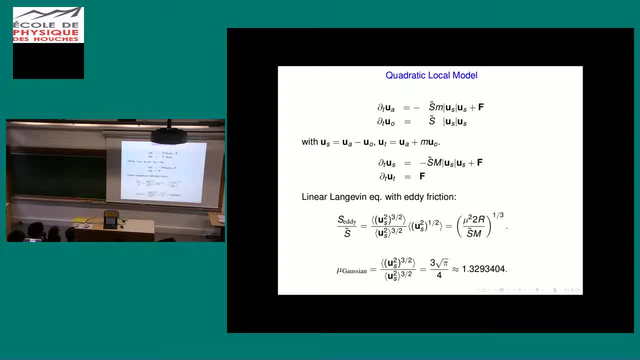 model, which is the linear model, by introducing an eddy viscosity. so the eddy viscosity can be calculated here explicitly: It's just U. It's just U to the power of 3 1⁄2 divided by the average of U to the power of 3 1⁄2,. 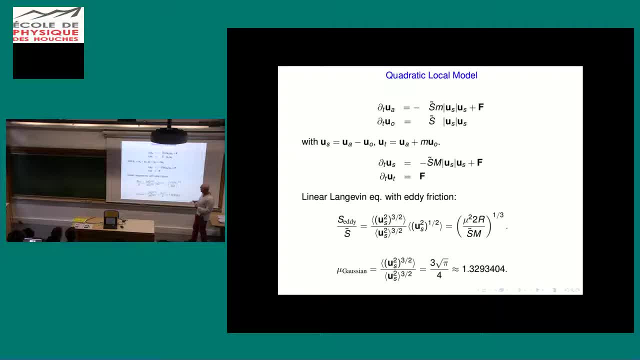 and times this value and you can give an analytic formula which is only depending on U, where U is given by this here. So this is normalized 3 1⁄2.. Okay, This is the moment of the square velocity and you can do the calculation. and if U, 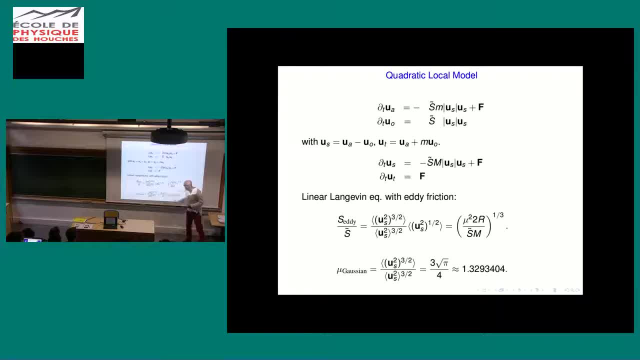 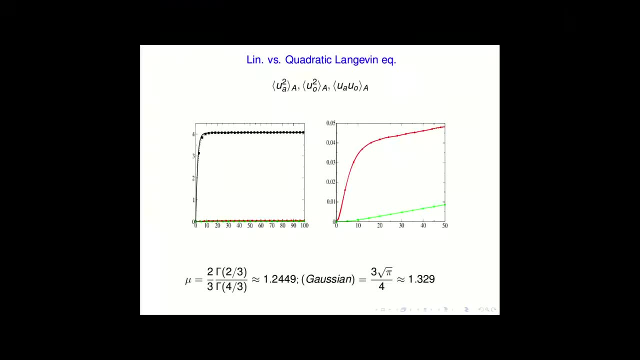 and V. the two components were Gaussian, then this would be just 3 to the square root of pi over 4, so something like 1.32, but in fact I managed to calculate. I'll talk about it. 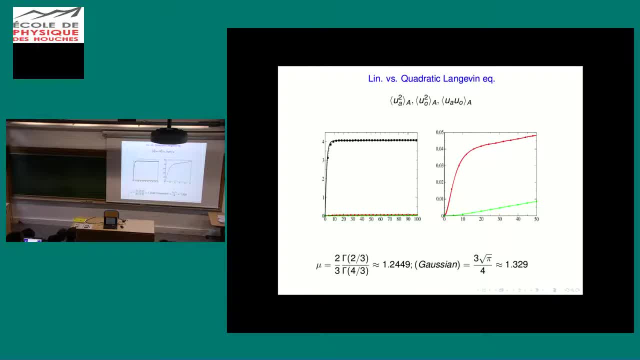 I'll calculate it. It's not difficult actually, as I found out. Okay, But the true value of U, which is just given here, where gamma is the gamma function. so it's the gamma function of 2⁄3 divided by the gamma function of 4⁄3 and 2⁄3 of this. 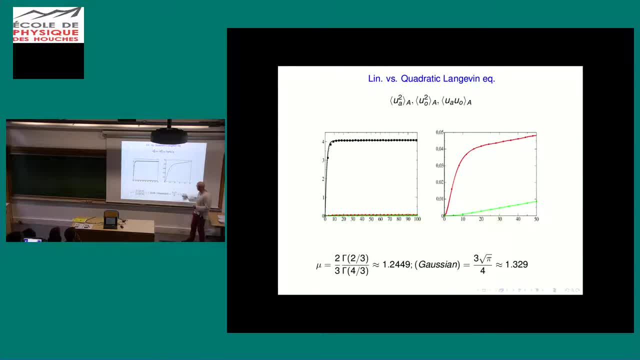 it's one point. so the true value is 1.25 something and this is 1.3, the Gaussian value. so it's not too different, but it's different. And what you see here in this plot for the zero-dimensional model, you see the integration. 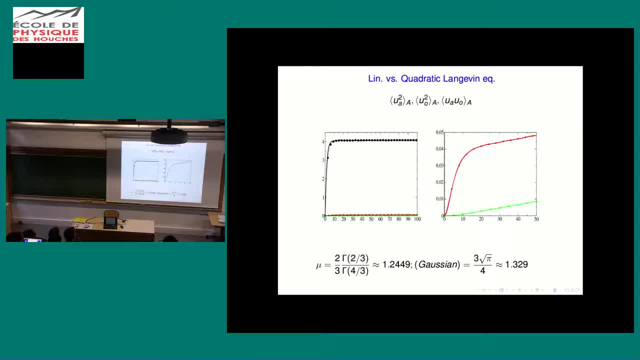 of Of Of. You see the analytic solution for the linear model, which is the dotted line here. So here you see a difference between the dotted line and the other lines. Then the symbols. here The symbols give the result of the numerical integration of the stochastic differential. 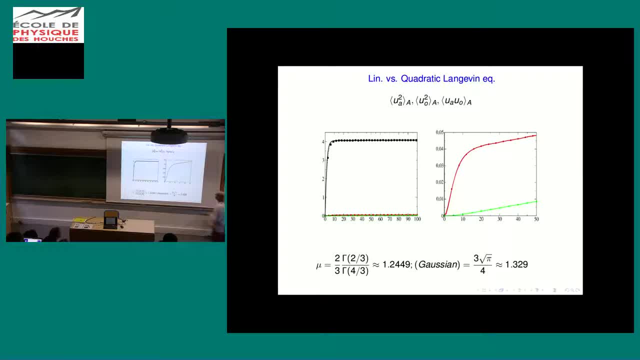 equation, the linear stochastic differential equation, and the full line gives the integration of the quadratic stochastic differential equation. So here you can see that this is the linear stochastic differential equation and the two lines here are the linear stochastic differential equation, and they both agree almost perfectly. 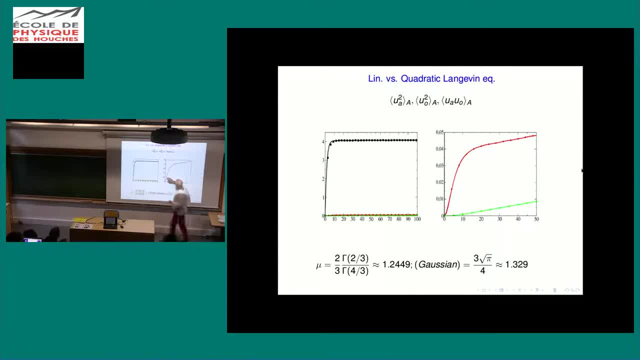 So in black would be the UA squared, red would be UAUO and green would be UO squared. And this is averaged over. I know this is averaged over many realizations. so this should be omega here, the A's should. 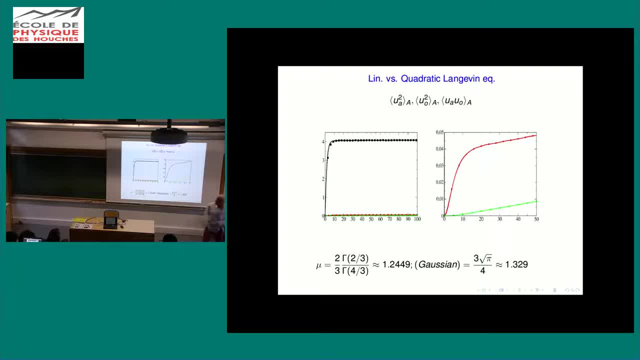 be omegas. It's averaged over many realizations. There's just a little difference in the beginning, In the build-up, In the build-up, In the build-up. But this is of course because this value here is only calculated for the stationary. 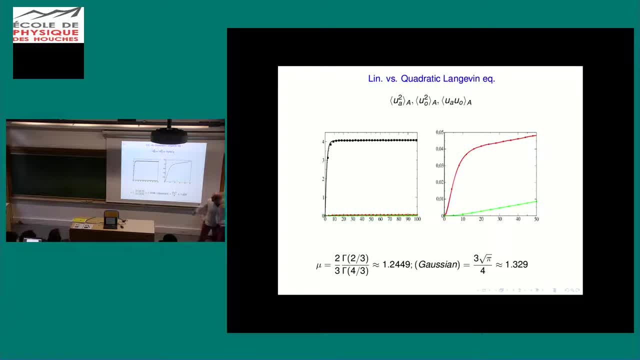 state For the spin-up this value is. I mean, it's different. I didn't do the calculation for the spin-up, just for the stationary state, And so things seem to agree There. of course, it's one-dimensional, zero-dimensional models, so they can be integrated with very 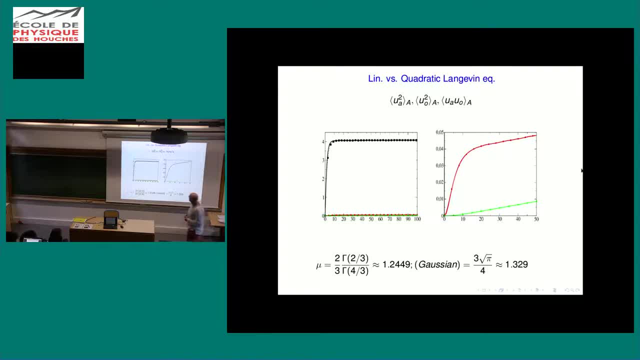 large ensembles. Ensemble size is always over one million. So this is why we disagree very well. So I just wanted to make a small parenthesis in two minutes left or so, How I calculated this value. Well, to calculate this value, actually, if you have the stochastic problems, you can. 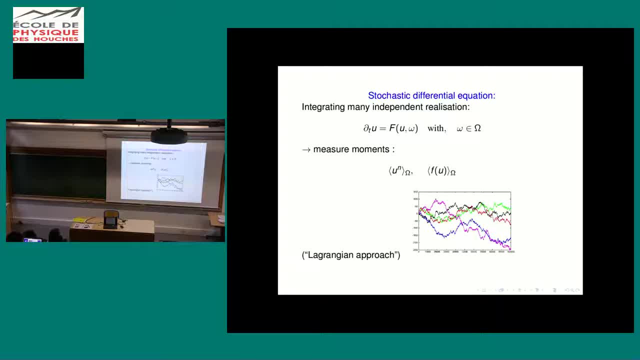 have two approaches to solve them. One is the stochastic differential equations, which I performed just like you start with a particle And for every noise, Realization of a noise, you do the integration And then, after some time, you arrive here. 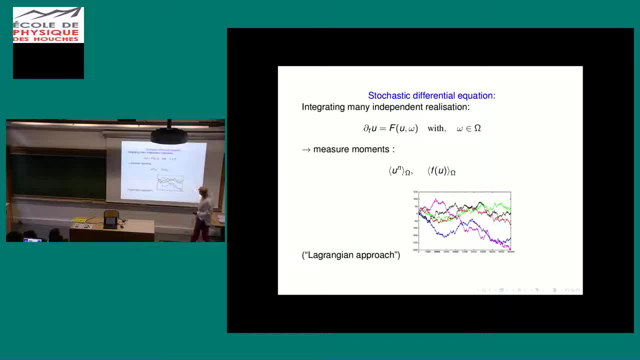 You do this for many particles- Here it's five, I've done it for many millions- And then you can calculate, you can make the statistics, you can calculate the averages or the moments, or you can also reconstruct the PDF. This is kind of a Lagrangian approach. 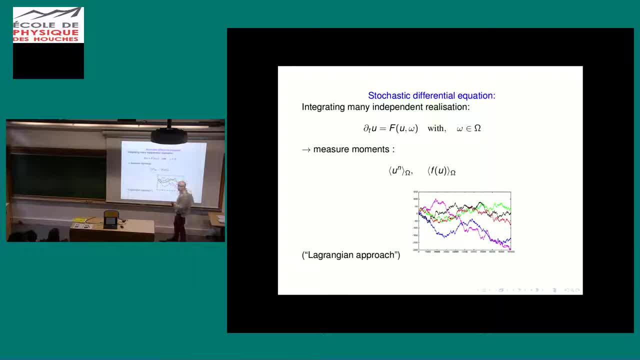 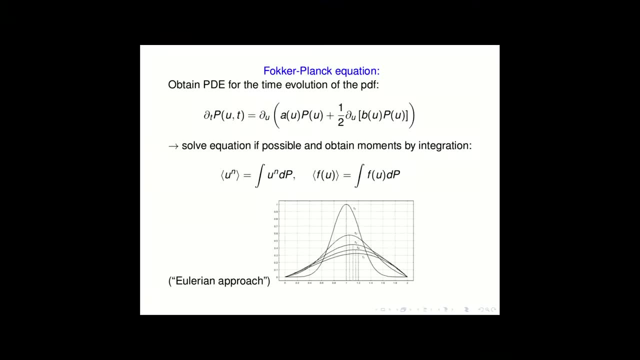 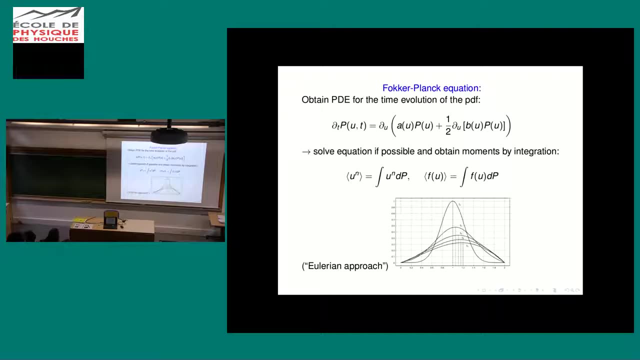 One could say this is a Lagrangian approach, because you follow every particle in this integration. You can also use- and this is actually more similar to what Albert Einstein did- you can use the Fokker-Planck equation. So in the Fokker-Planck equation it's different, because you try to write down an equation. 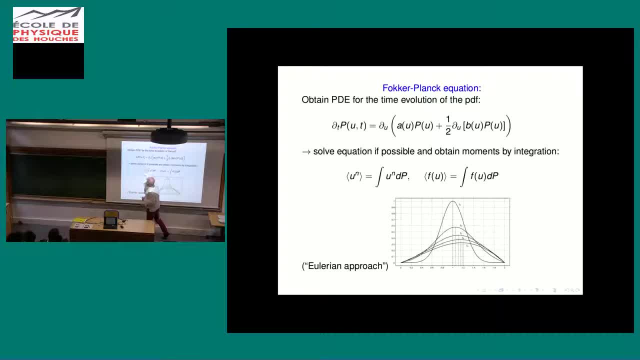 for the PDF, the probability density function. You write down a partial differential equation and then you see how it evolves, So how this PDF, this PDF here, moves and how it spreads. This is given by this Fokker-Planck equation. 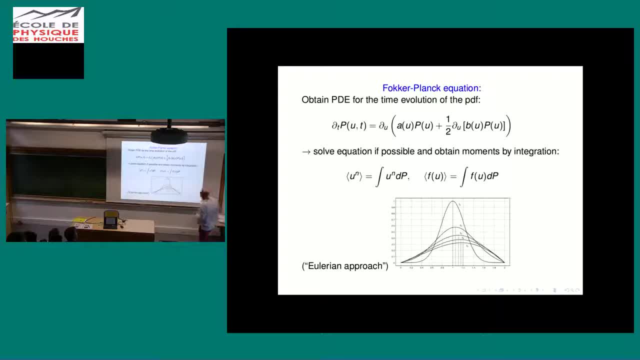 It's kind of an Eulerian approach. So I mean would be. I mean, is everybody familiar with this? or you want me to explain in two minutes? Maybe I explain it, or yeah. So if you have a, if you, for example, want, if you have particles which are moving around, 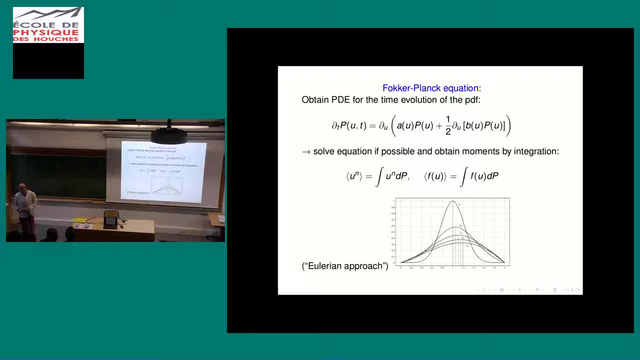 and you want to know how many particles are in a square like this, then you can just look at all the particles and into or have many particles, Identify them, and then at some are moving out, some are moving in and then at one point, 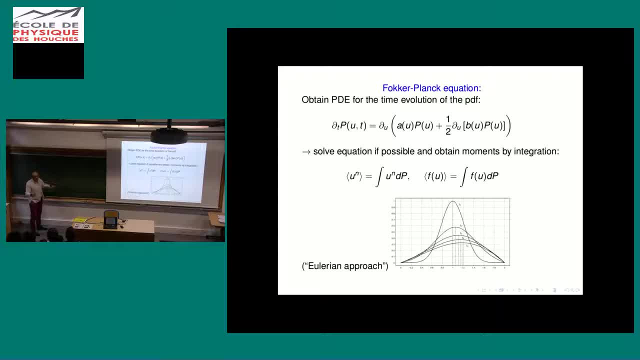 in time, you stop and you count how many particles are there. So this would be kind of a Lagrangian approach, because you follow the particles how they are moving. But you can also write an equation or try to find an equation: What is in a at a certain time? what is the probability of a particle from this here to? 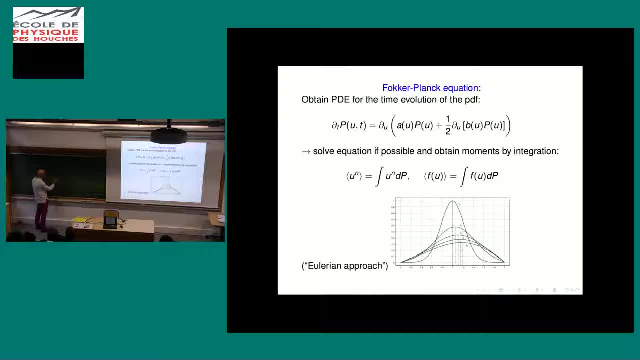 jump in here, from here to jump in here and from here to jump out. And so this would be the Eulerian approach, the Fokker-Planck equation approach, where you just look, you just write down equations, how these evolve. so how is the probability? 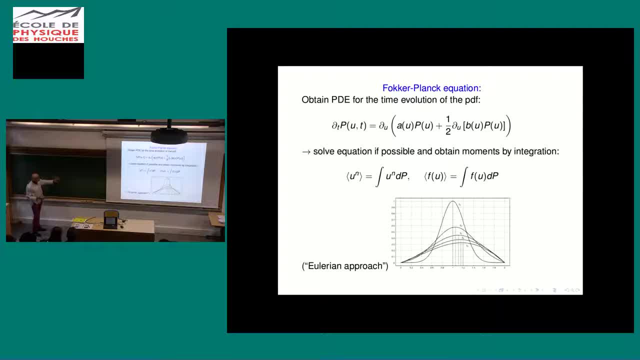 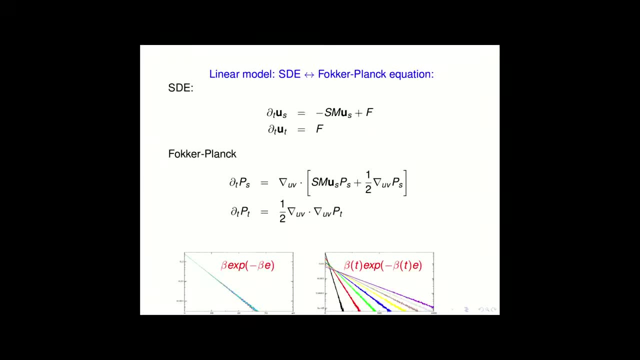 of a particle jumping in or jumping out, and then you get this approach. So you have these two approaches and four of my simple models. then what you have is: you have, you can write down the stochastic differential equations you can write down: 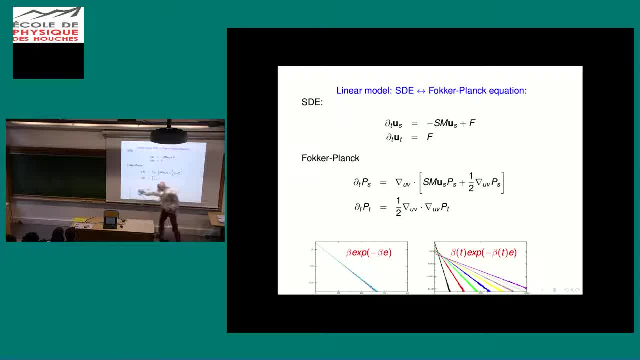 the Fokker-Planck equations And here I compare the two. so it gives us: this is a comparison of, and they all fall on the same line because of course my ensemble sizes are so big And I could also do this for the nonlinear model. 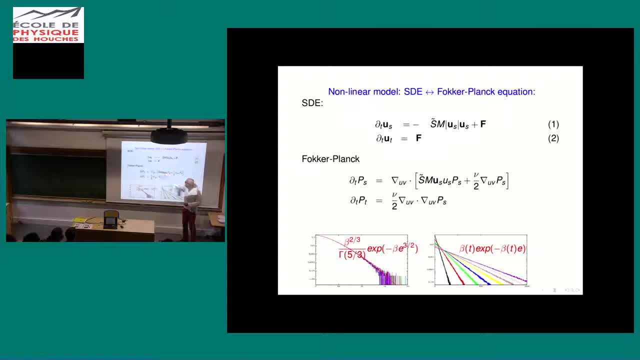 where you have. this Fokker-Planck equation is given here and you can solve it. and if you solve it, you find out that this is this, where e, e, here is now u squared plus v squared, and so it's just exponential to the power of minus beta, to the power of e. 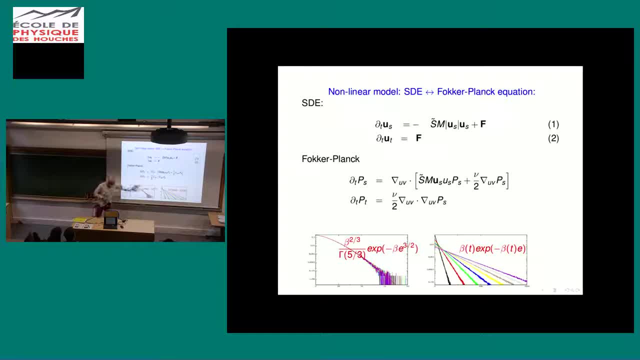 or to the power of three-half, and then there's a normalization factor which depends on the, which includes the gamma function. So we have these two approaches and I just wanted to show this because it the red line. the red line is the Fokker-Planck solution. 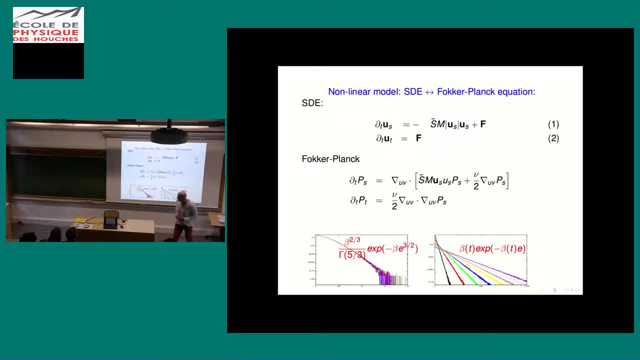 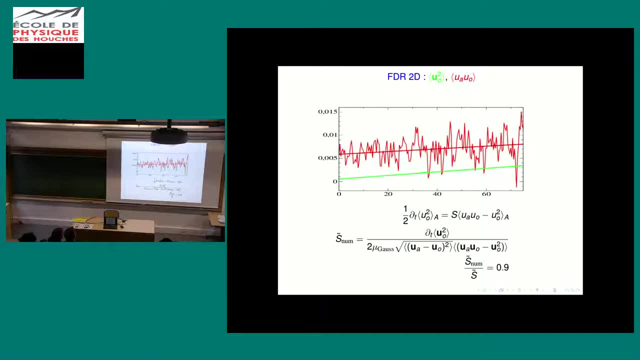 and the other Wigley lines are actually the integration. so there's perfect agreement for that. And so this is my almost my last slide, because I go back to comparing. I mean, now I go back after having spent some time in zero-dimensional space. 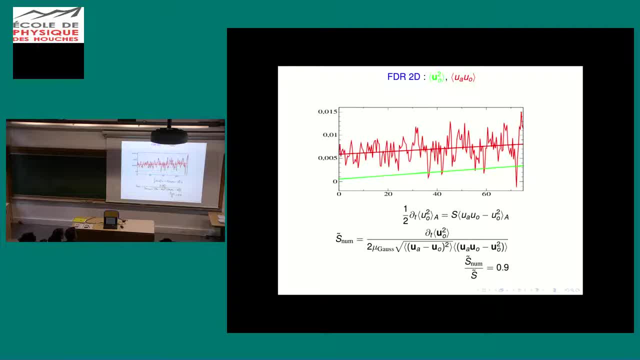 I go back to two-dimensional space. This is the picture you all have already seen, where you have the correlation a- u- o and the correlation autocorrelation of u- o, and what you see is you can take the gradient out of this. 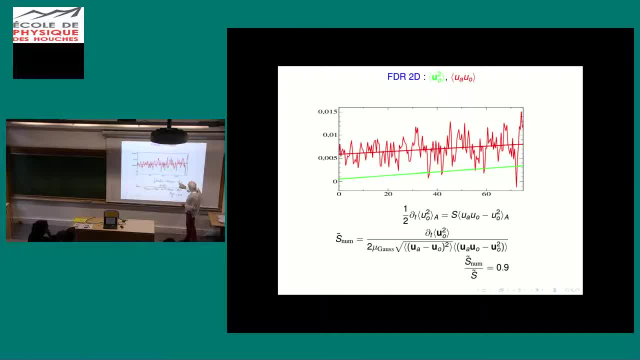 you can calculate. you can calculate the u a, the u o and the u o squared, and you can use this. so here I used the linear Fokker-Planck equation and also the linear the equation for the stochastic differential equations. 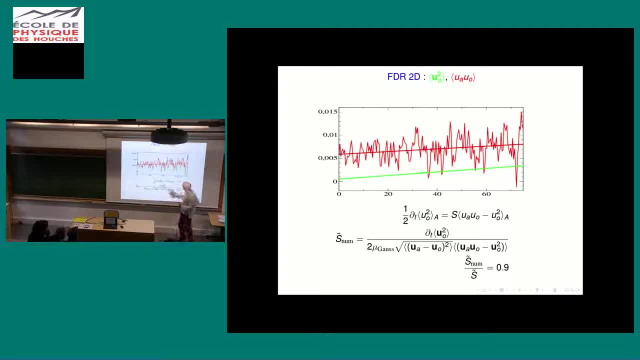 and I can obtain. then, by just looking at all these correlations, I can, I try to estimate the, the friction, the eddy friction coefficient, and of course I know it. no, the friction coefficient not eddy, but just the friction coefficient. 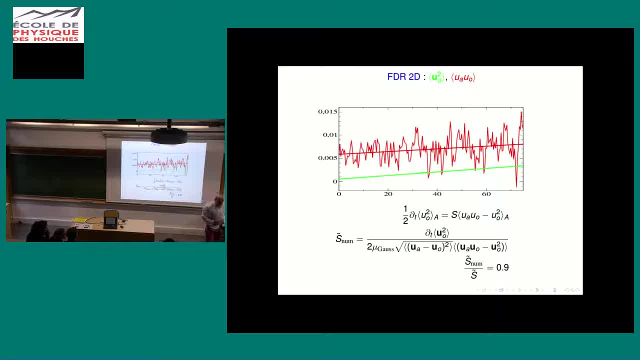 and I know it, and it's close to the observed value. Yes, please Excuse me, could you remind us what beta was in the slide before this? It's just a constant. It's just a now be sure, It's just a constant which is evolving in time for the 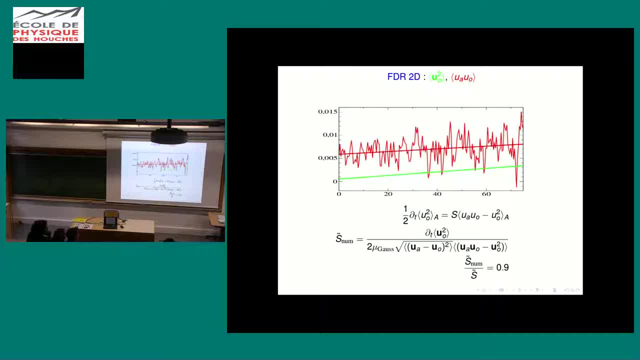 for the total mode, because it's a diffusive process, and for the shear mode it converges to a, to a, to a value, to a constant value. So this formula that you showed, beta to the two-thirds exponential, and so forth. 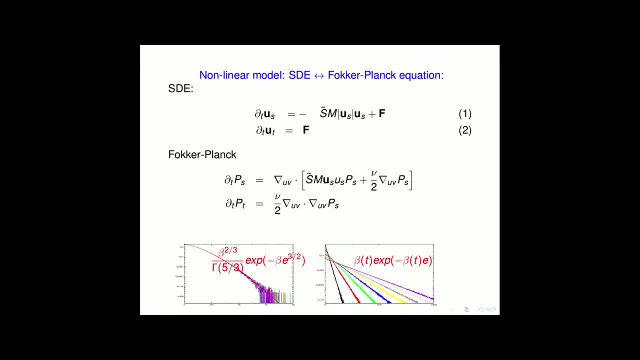 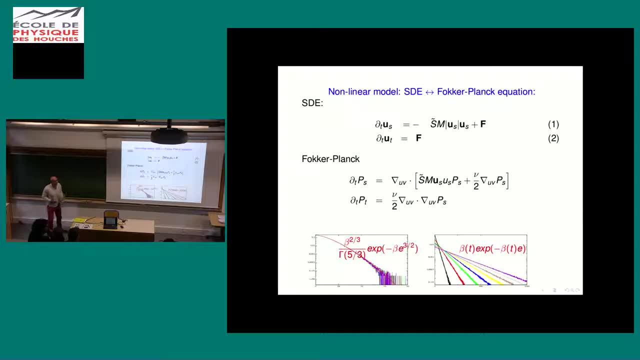 that was the probability distribution. or This is the probability distribution for, for, e, for this quantity, for the, the energy I mean, And that you get by solving the stationary for? Oh, you just have to find the stationary. 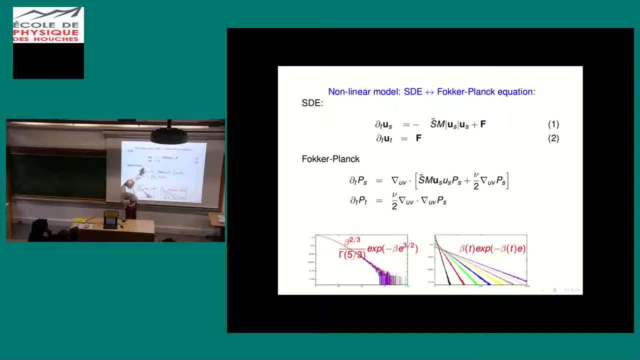 stationary, stationary. You have to just have to find the solution. You put this zero and you find the solution of this, And so then you, you have it. It's actually not how it happens. How it happens is you do the experiments. 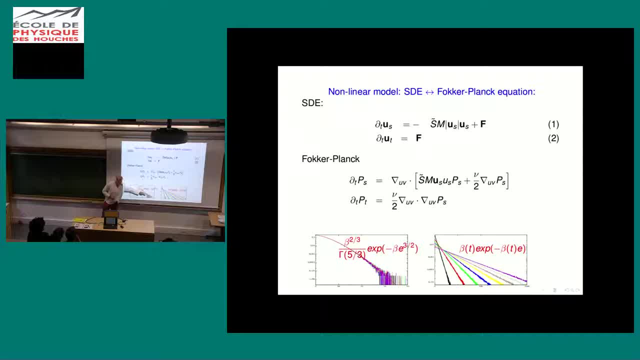 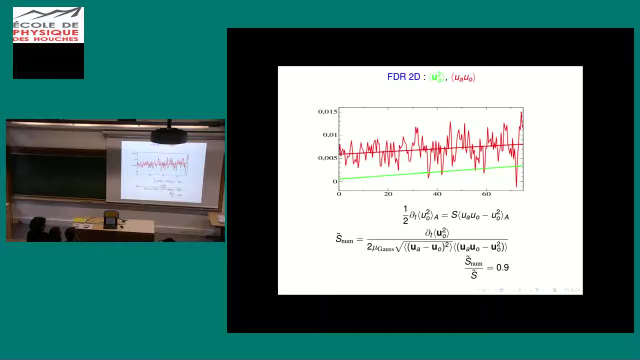 You find that it, you find that it gives a certain law, and then you try to fit, and then you take your fit, You put it in the equation and it works. Voila, Okay. So so the, the, the, the method works very well in estimating, or. 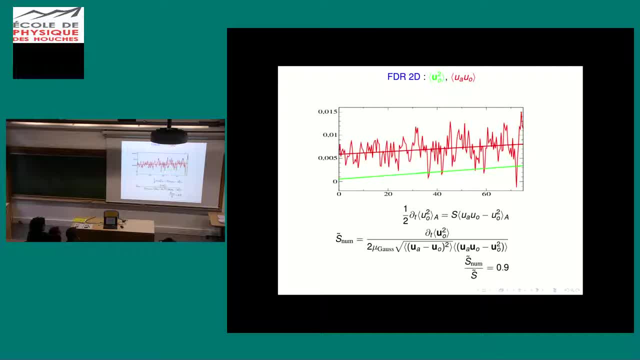 or finding the, the, the, the surface friction, And so it can be applied to some extent to the two-dimensional simulations. And this is where I'm about for the moment. I mean, I have other results of course, also about the estimation of m and the other values in the problem. 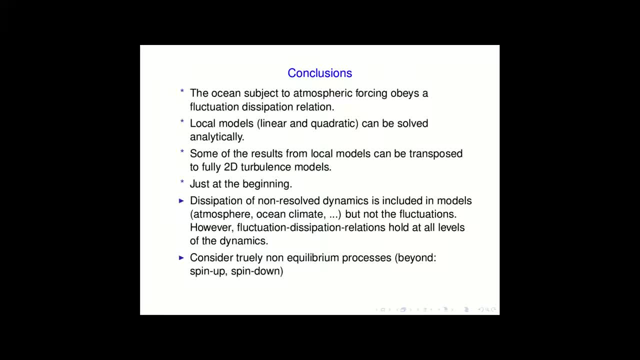 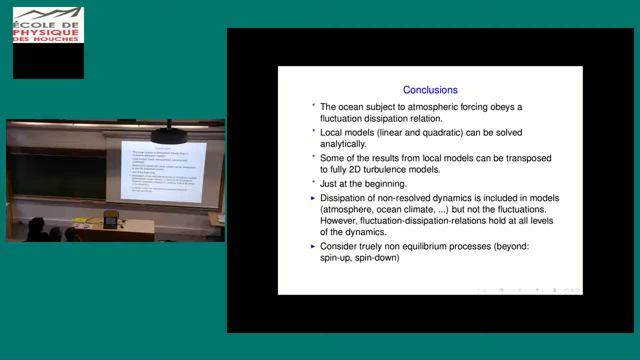 And to finish, I just conclusions, make a few comments. So the first thing is that the ocean subject to atmospheric forcing obeys a fluctuation dissipation relation which I have written down. for this, zero-dimensional models, The local models, linear and quadratic- can be solved analytically. 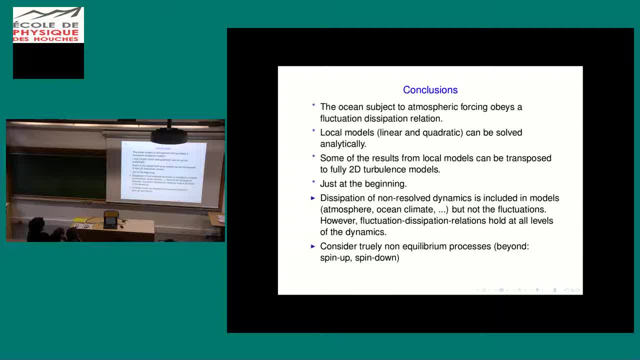 We have analytic solutions of them. Some results from the local models can be transposed to the fully two-dimensional turbulent Models. what I wanted to say is: it's just the beginning, And then I have two kind of comments. The one is that it's, it's, it's. it's larger than what I'm presenting now. 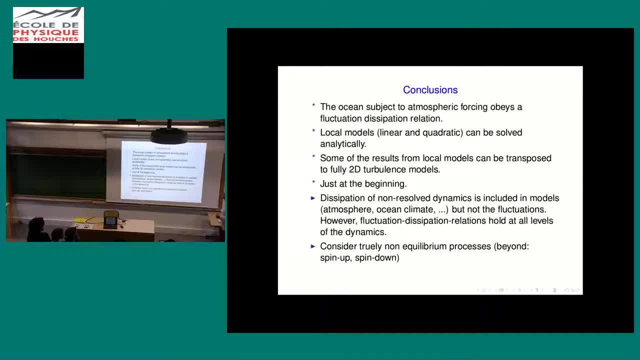 but I mean, it's just maybe for discussion that today the dissipation, the small-scale structures which increase the dissipation of the system, are always included. the dissipative effect of the small-scale structures is included in the atmosphere, ocean and climate models, but not the fluctuations. 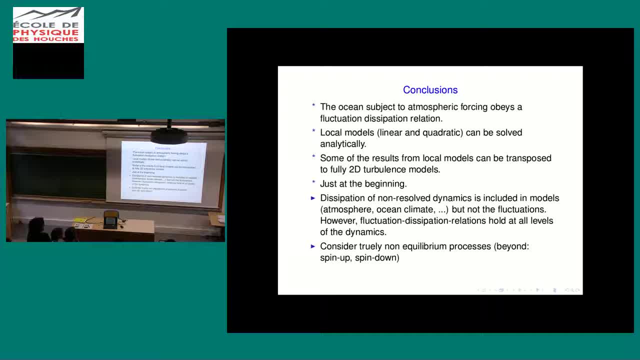 But we have fluctuation-dissipation relations at all levels in the dynamics. So if you have kind of a Laplace operator to take out the energy, we should. we should also have something which kicks a little bit the system, And for this of course you have to have to have to write down the 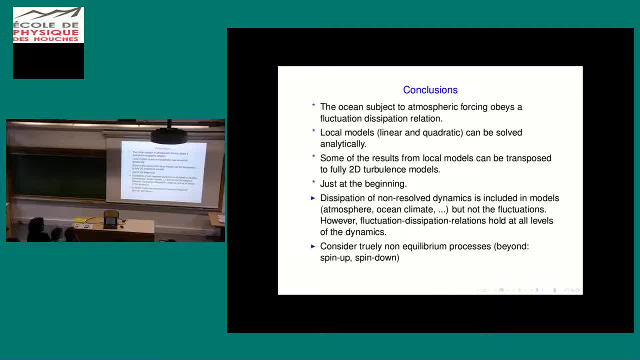 we have to find the fluctuation-dissipation relation. So The bows have the nice, the good magnitude, so they have to that they correspond to each other. And I recently heard that some people who do weather forecasts they say that often weather forecasts work better if you do the calculations in single precision rather than double precision. 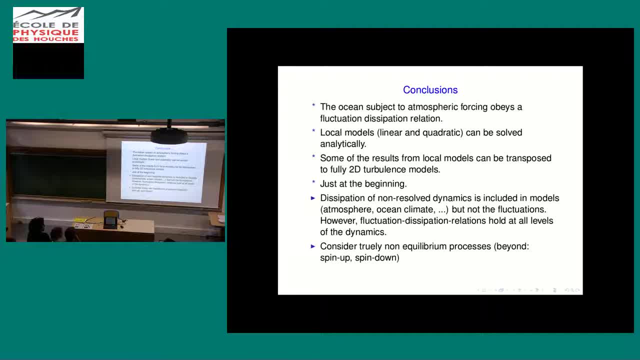 And I think this is a manifestation of the dissipation-fluctuation relation, because if you have single precision, then you include some kind of noise which also kicks the system, And so you have dissipation and fluctuations. but then I think it should be done more precisely. 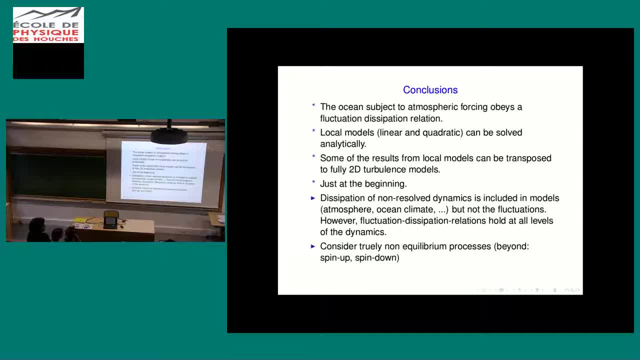 more qualitatively in developing the fluctuation-dissipation relations Between the two, And then I consider a truly non-equilibrium process. so it's a process which is evolving, so I cannot continue my experiment forever, because energy increases, increases, increases. 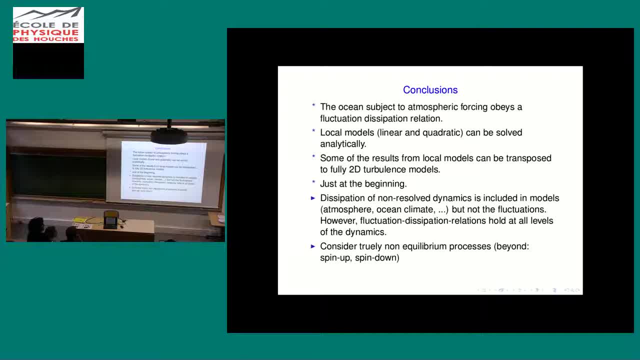 But I think this is important today, that we go to this really non-equilibrium process, not only spin up and spin down, because I mean we have a certain forcing. the system spins up but before it reaches equilibrium, I think the forcing- the weather system or what forces it has already disappeared- has already changed. 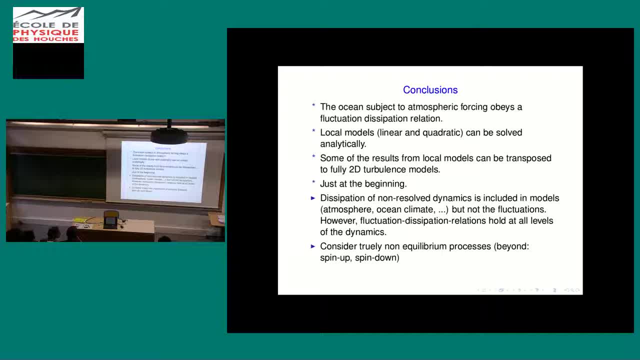 So I think this truly non-equilibrium process are very important and should be also considered because forcing functions also vary in time and often the adjustment to the forcing, the spin up, is longer than the presence of the forcing. So this is the 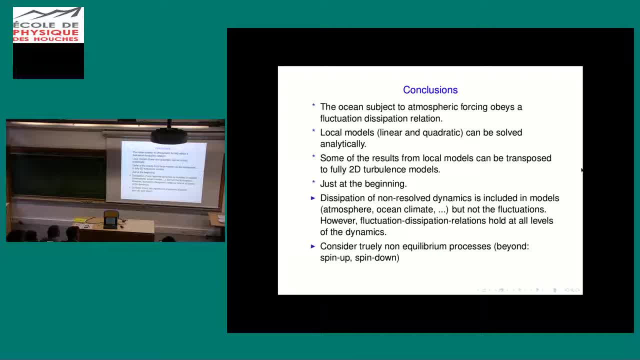 This is the end of my talk and I'll be very happy to take your comments questions. Thank you. So can you hope to also have in observation a kind of signature of this relation? I hope, yes, Probably it's. I'm not at all a specialist of the genesis of cyclones and anticyclones. 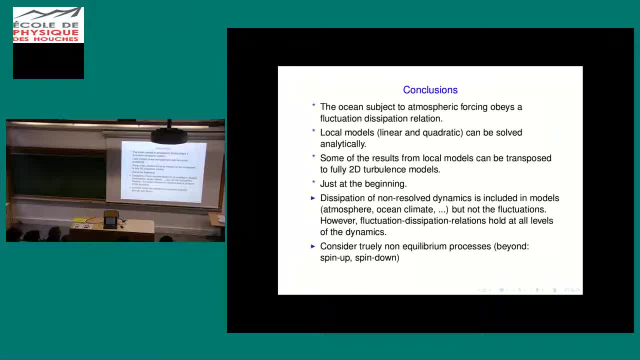 but I've heard, or I've read, that in the initial phase the motion of the ocean could be important in this case. So If you have an ocean eddy, it might attract an eddy above an atmospheric eddy, A cyclone, an ocean cyclone can attract an atmospheric cyclone. 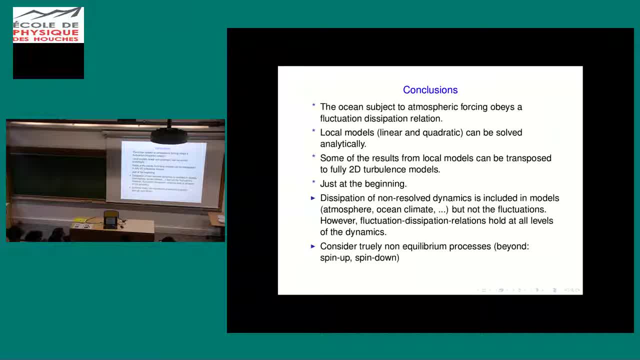 have a condition which favors atmospheric cyclones, not only by thermal exchange but also by exchange of momentum, And this might be interesting to consider, but I mean, I haven't gone so far. So, in general, when you have systems with two very different timescales, 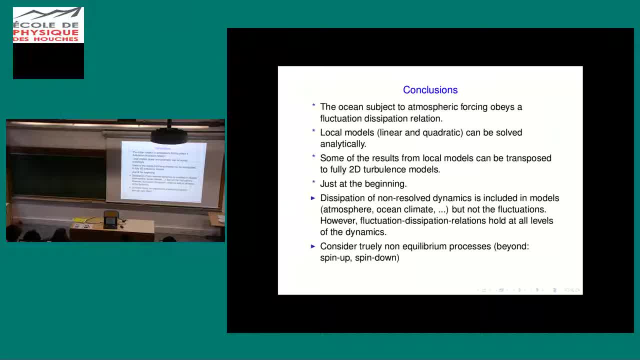 when you look at the effect of the fast system on the slow one. so you get at leading order an average effect, and then you get at next order a white noise which amplitude is given by a cubo formula. So it's basically roughly the variance multiplied by the correlation time. 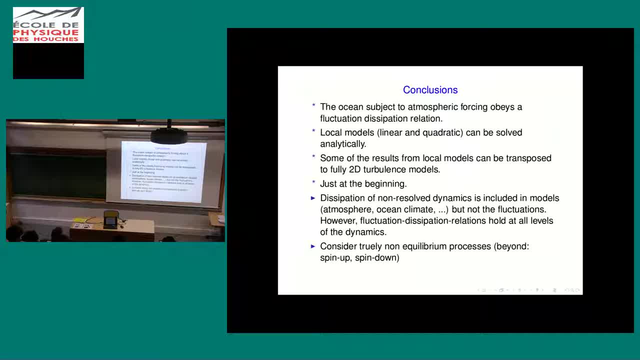 but gives you the value of diffusion coefficient in front of it. So I wonder how what you discuss is different from this. I don't know. So what happens very often is that the average is way larger, For instance for the real atmosphere acting on the ocean. 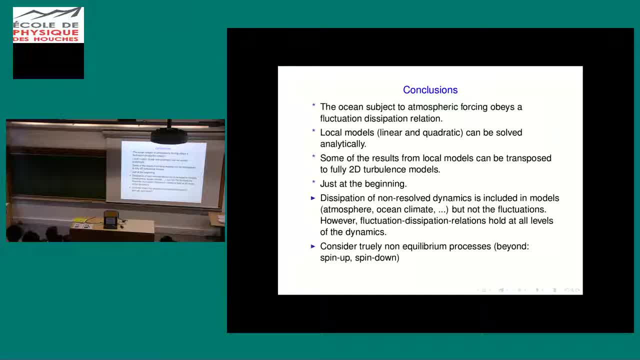 you have the average wind, So you have. You have the average wind, and then you have the fluctuation. So one would like to compare the typical effect of the average compared to the effect of the fluctuation, for instance from the point of view of energy. 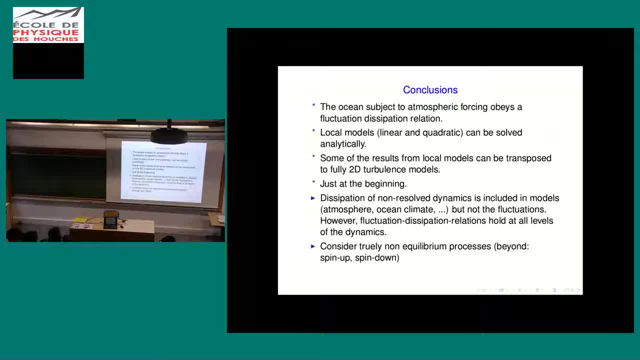 So in my case, for the moment, I do not have an average wind. I mean, the average wind is zero. I don't know how this applies to what you're saying, So I'm not sure to have understood why the two couple systems. 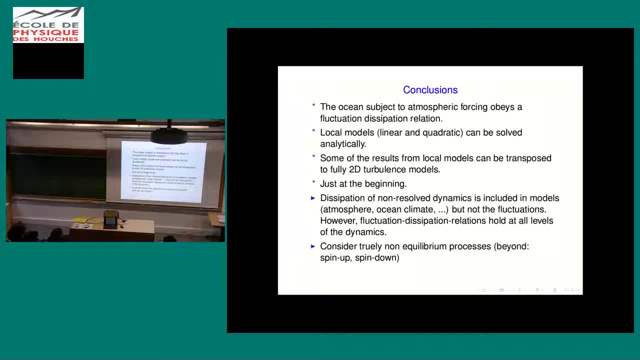 don't have at all the same time scale for their evolution, because if we assume that there is a very rapid excitation at the surface of the ocean, so even if it's very small, you could have small amplitudes, small-scale forcing, which would end up with the inverse case. 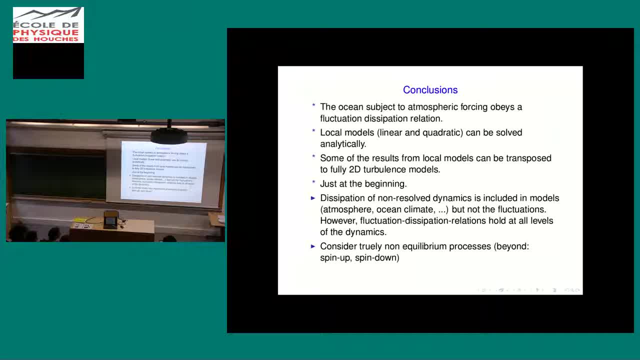 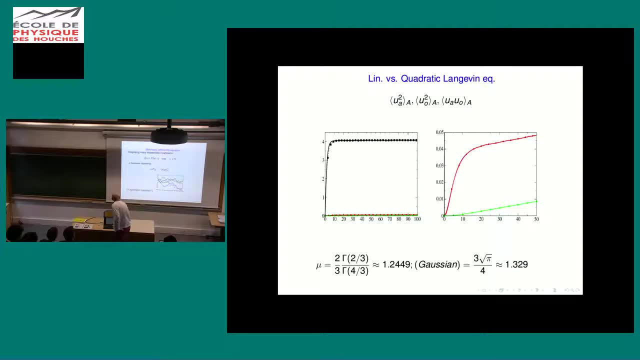 gain in large-scale motion at the same speed. So I don't get why there is this discrepancy in time scale. So in the linear models it's clear, because I mean, the mass of the ocean is just so much bigger And so if you just look at this equation, 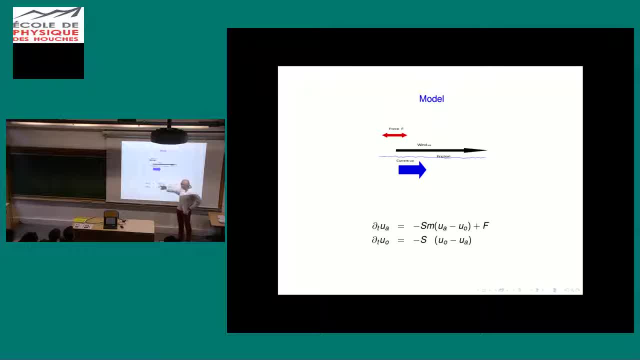 so this is kind of the inverse. This is the inverse of a correlation time. And then you have here you have a factor of 100, right, So it is very different. So locally it's clear that it's different. Afterwards there's the problem of the cascade. 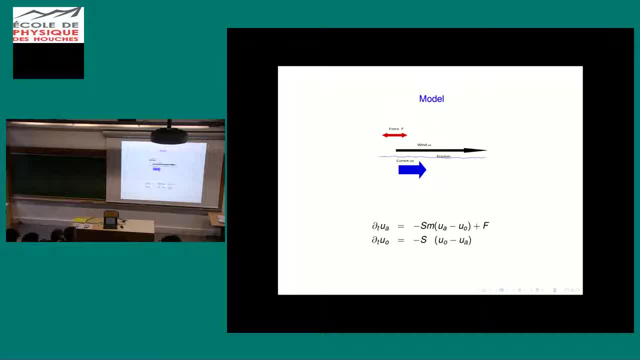 the energy and the entropy cascade, And something which I have not said is that this, actually, why do I need in the two-dimensional model? why do I need 4,000 times 4,000?? It's because, if this for this to be true, 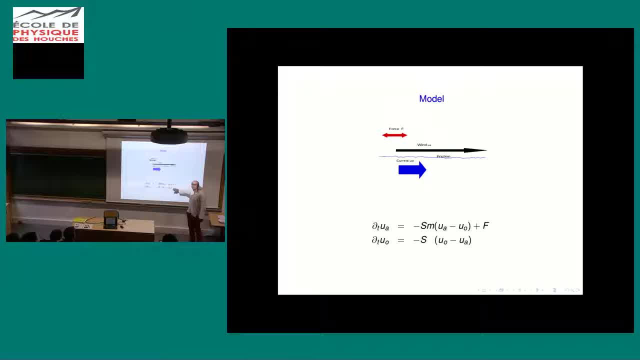 I do not have, I'm not allowed to have dissipation here, another kind of dissipation of energy, And if you, if the ocean model doesn't have enough resolution, then there is too much energy dissipated, But in two-dimensional turbulence.